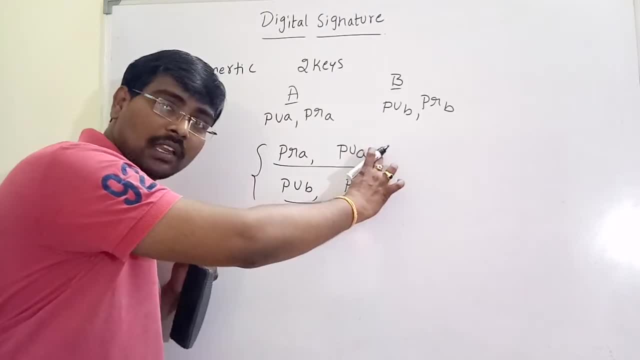 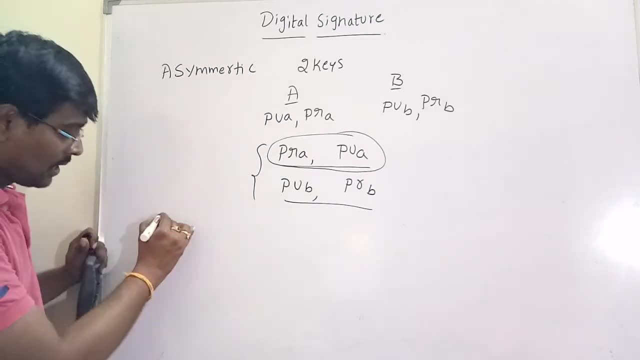 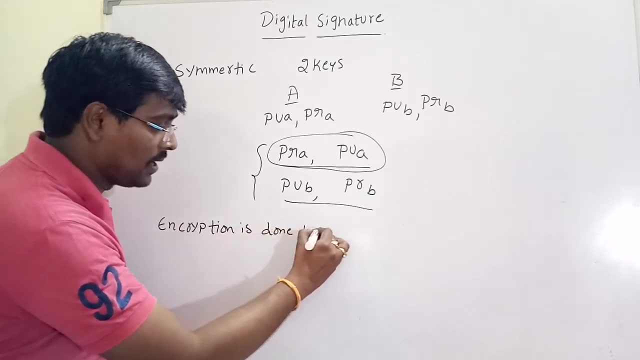 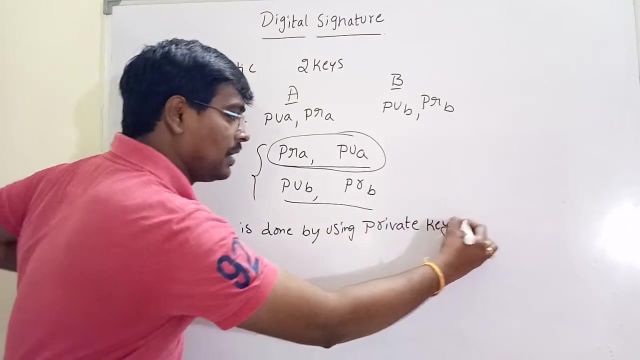 we are using the same set of keys, That is, the keys of either A or the keys of B. In this, this one is called. this one means encryption is always performed at the sender side. Encryption is done by using private key. Encryption is done by using private key. 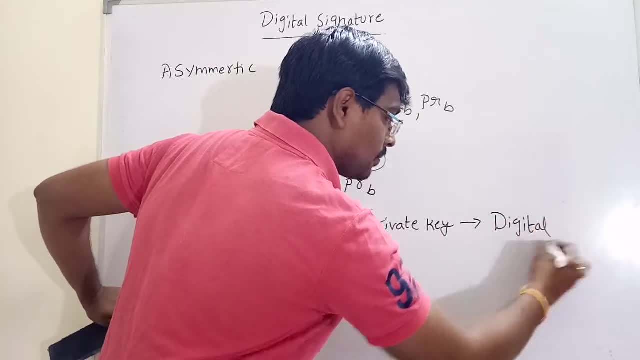 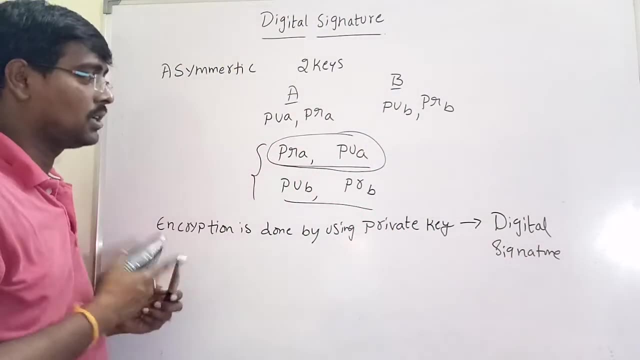 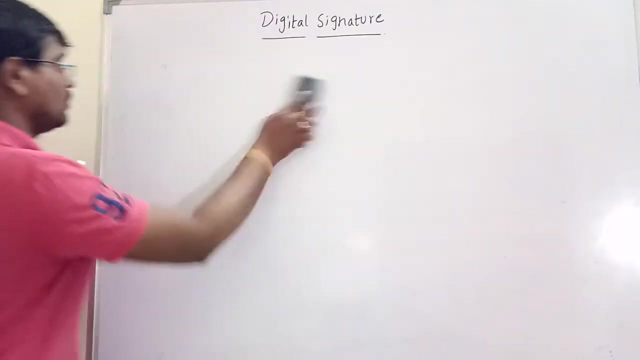 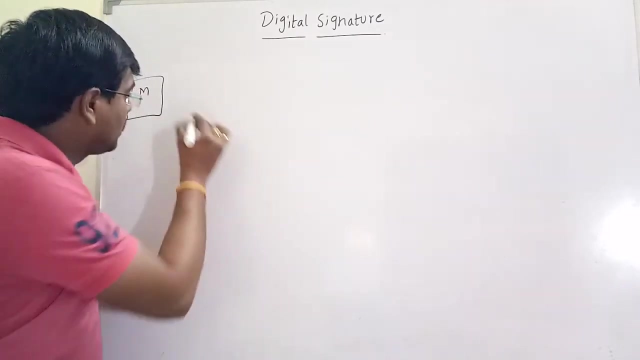 It is called digital signature. What do you mean by digital signature? Encryption is done by using private key. It is called digital signature. Suppose: see the diagrammatic representation: M is the message. Suppose: M is the playtest. For this playtest, I am applying an hash function H. 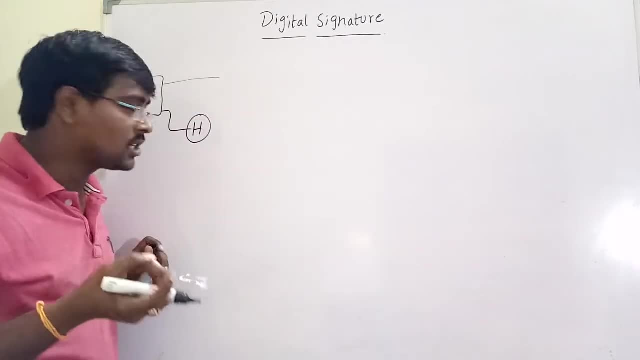 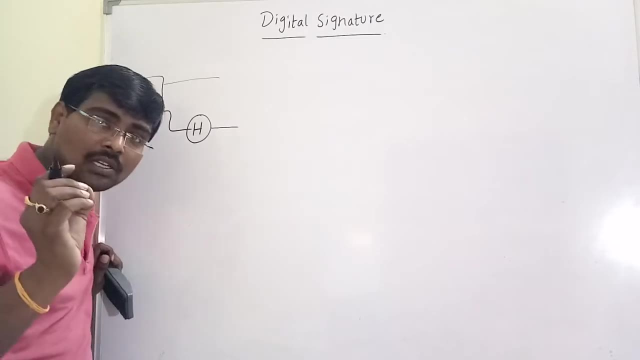 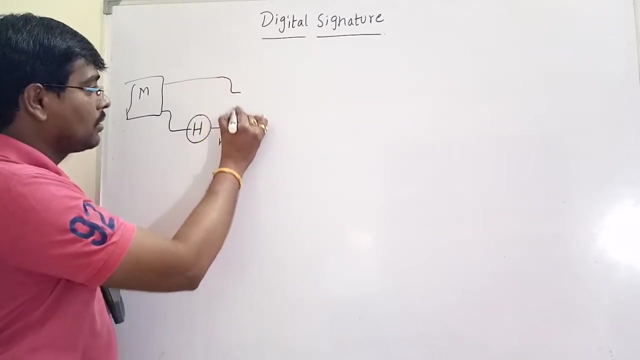 H is any hash function That is either SHA-1, SHA-512 or HMAC- any hash function. It produces some hash code. H: after applying H, it produces some hash code. For this hash code, I am appending this one. 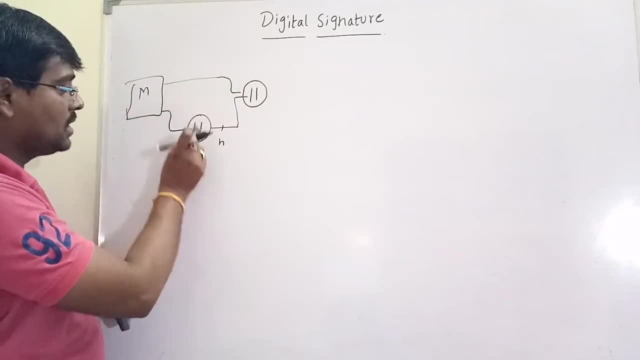 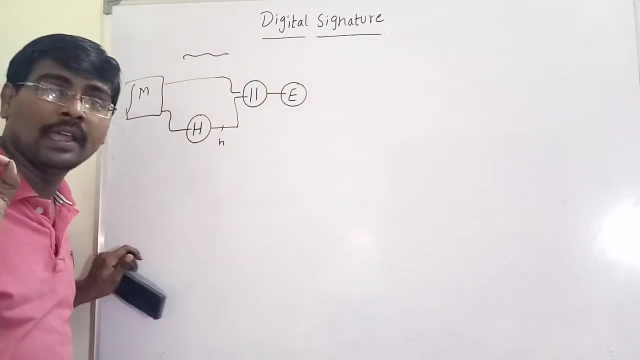 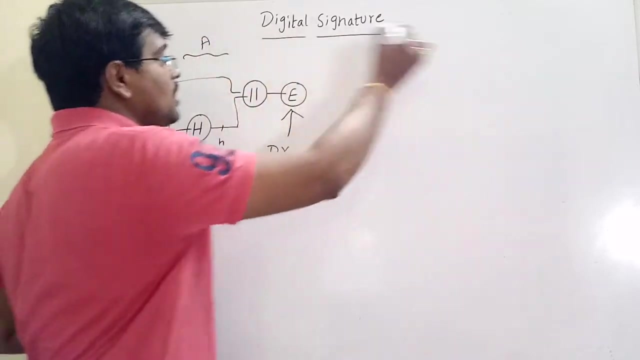 The symbol is appending, So I am appending the message with hash code and perform encryption. Suppose this is at the sender side and perform encryption by using private key of H. Suppose the sender is A, The receiver is B. By performing encryption with private key of A: what it produces. 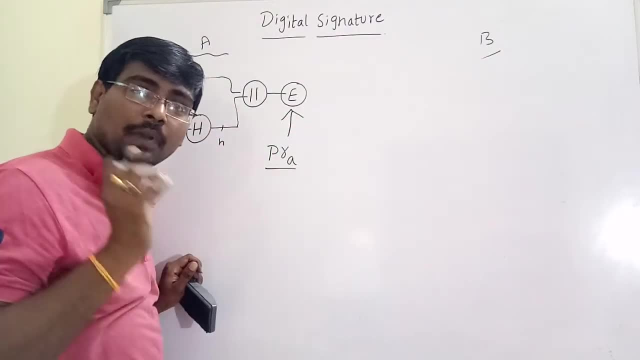 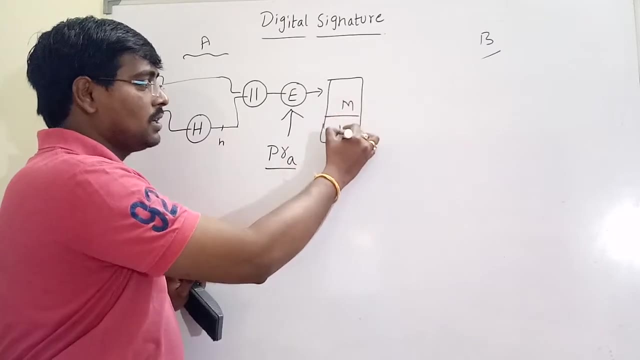 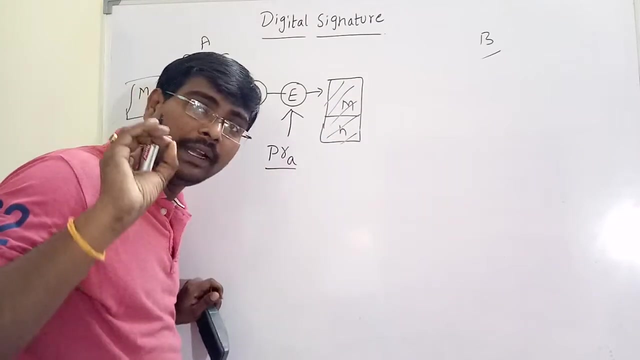 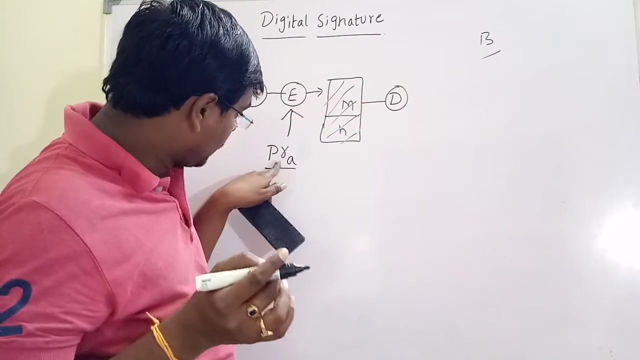 It produces the message and hash function H. The message suppose, And what we will do: Apply decryption at the receiver side. Suppose, by applying decryption at the receiver side, if you are encrypted by using private key of A Compulsory, we have to decrypt using public key of A. 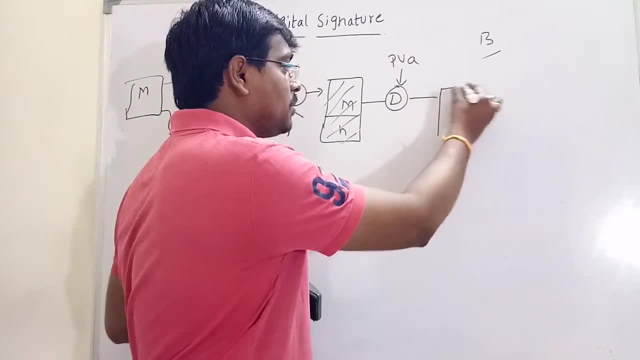 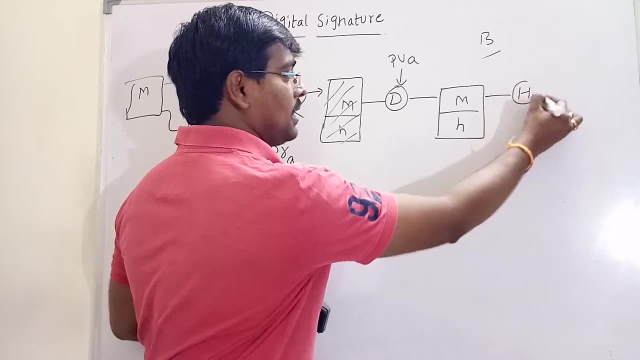 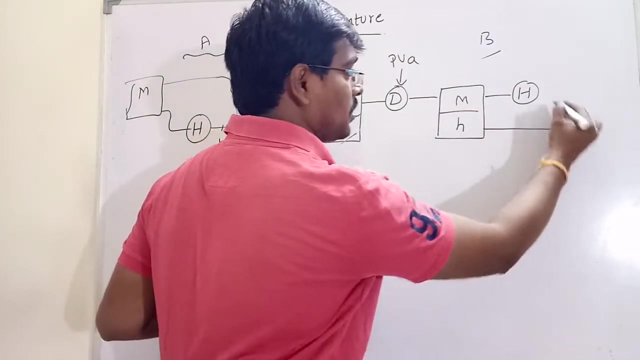 Decrypt using public key of A Suppose it produces. After decrypting, it produces M and H On M. apply the same hash function is Whatever the hash function we are applying at the sender side. apply the same hash function and compare both the results. 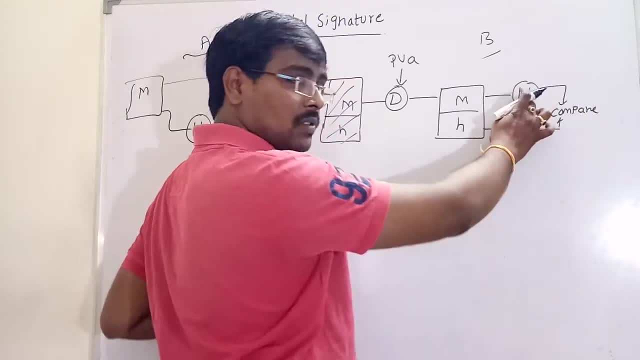 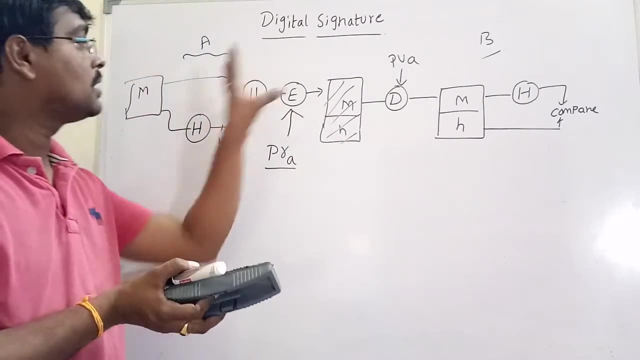 If these two are same, That is the result of this hash function. That is the result of this hash function and this hash. If both are same, our encryption and decryption is performed successfully. This is jigsaw signature, Remember. the only point is: this is the sender side. 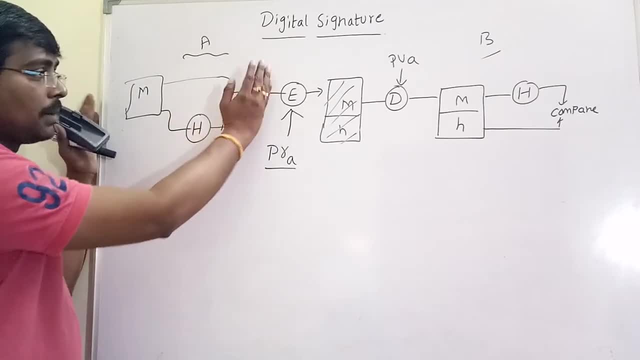 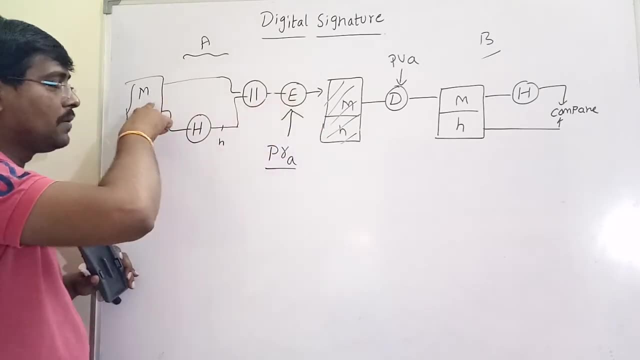 Whatever the operation we are performing, that is encryption. The encryption is done by using private key. If the encryption is only for the message, or if the encryption is only for the hash code, or if the encryption is a combination of it. whatever happens, this is not the case. 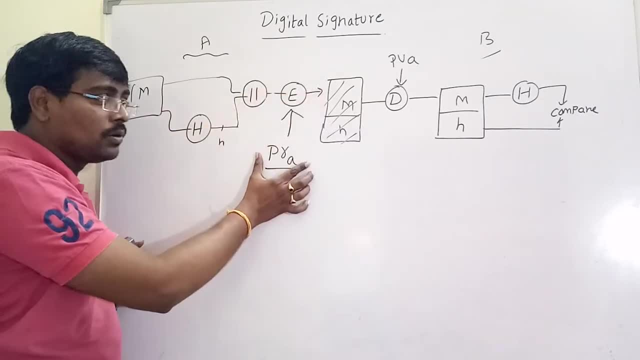 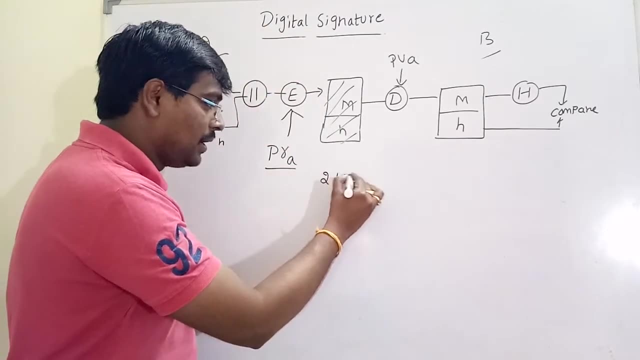 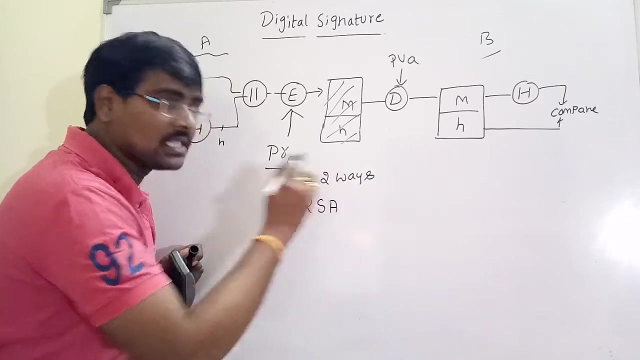 The encryption is performed by using private key. This is digital signature. Now, the digital signature is implemented in two ways. Digital signature is implemented in two ways. One is RSA approach. We already know RSA algorithm, So here encryption is performed by using RSA algorithm. 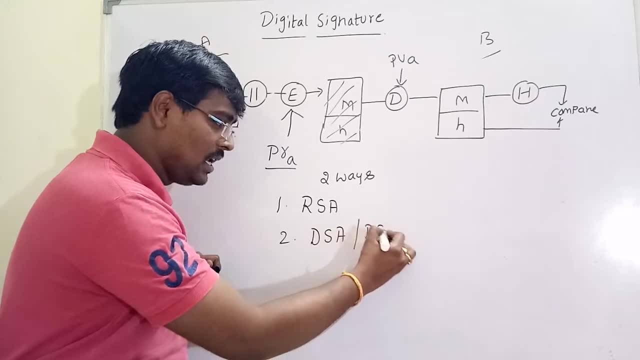 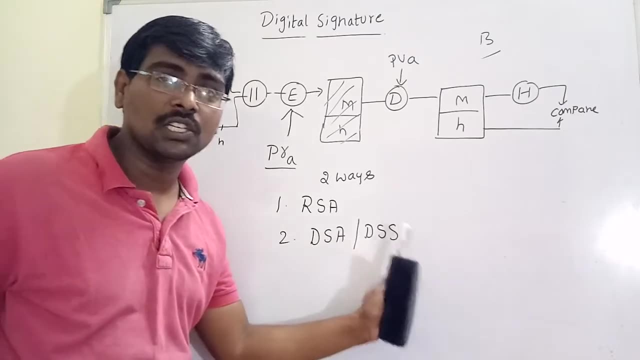 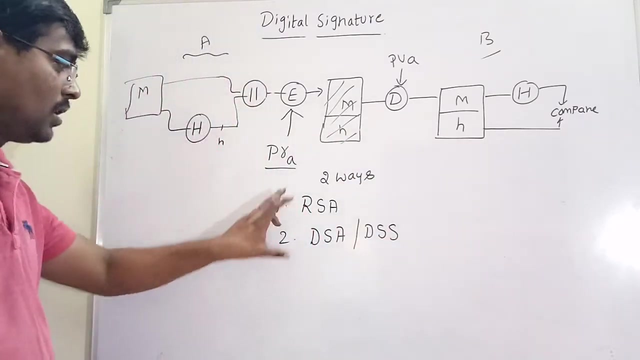 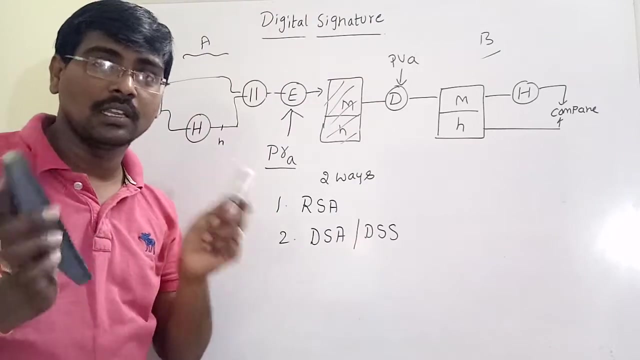 Second one is DSA or DSS approach. DSS is digital signature algorithm or digital signature standard. Both are same. Remember: digital signature algorithm or digital signature standard. Both the terms are same. By using any of these approaches, By using these two approaches, we are performing the digital signature concept. 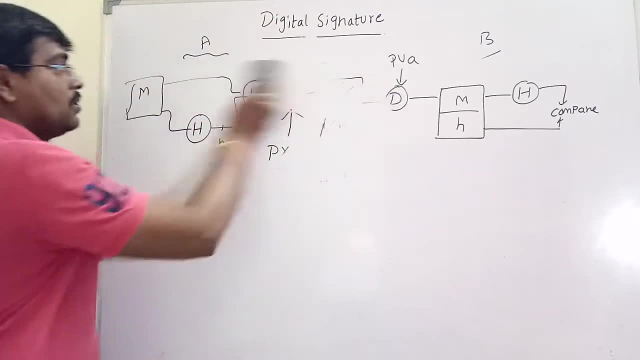 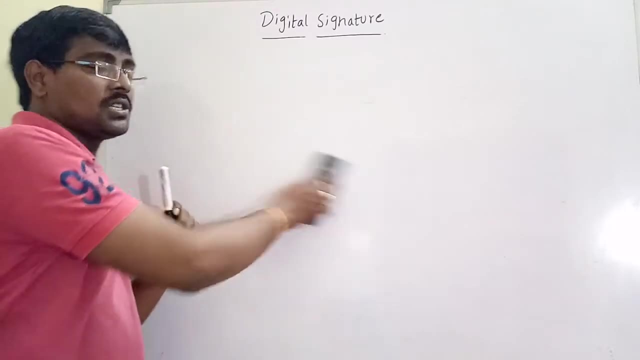 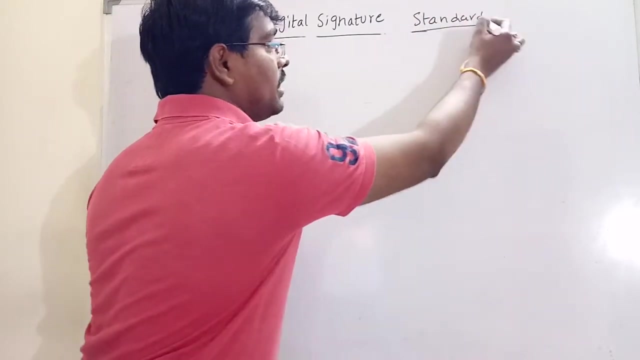 Now first move to RSA approach. This is a very simple approach, Only a single diagram. We will clearly discuss digital signature. Remember, our concept is digital signature standard. We have clearly discussed DSS approach. First move to RSA approach. 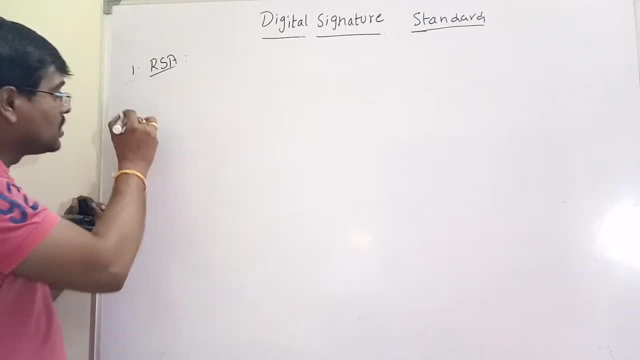 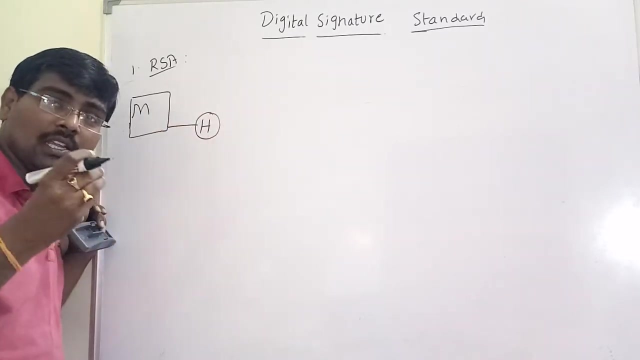 First move to RSA approach. The procedure is very simple. This is the message Here. M is our plain test For that message. I am applying some hash function H Here. we already discussed it. Hash function is any SHA algorithm. 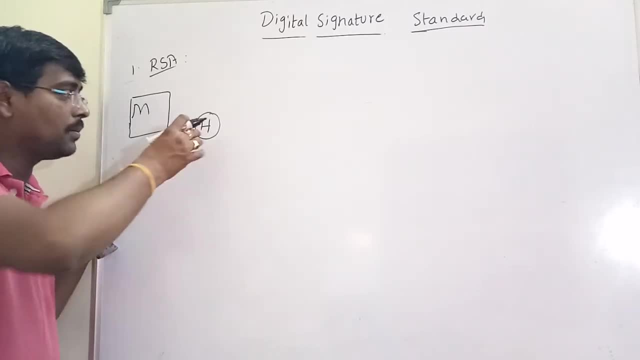 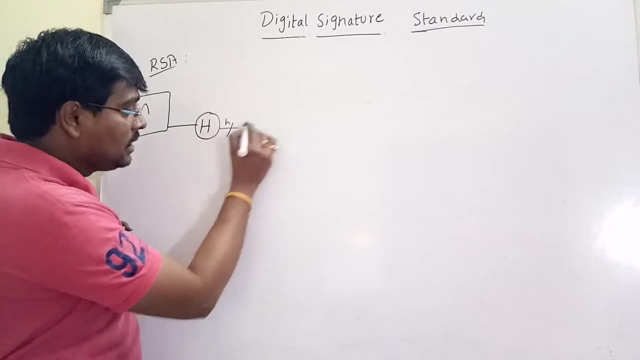 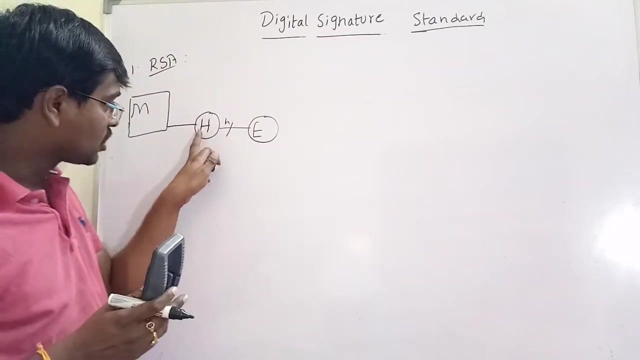 Either SHA-1 or SHA-512 or MD-5 algorithm or anything. Apply some hash function, It produces some hash code. On this hash code, I am applying encryption. Remember, in RSA approach for this hash code, I am applying encryption. 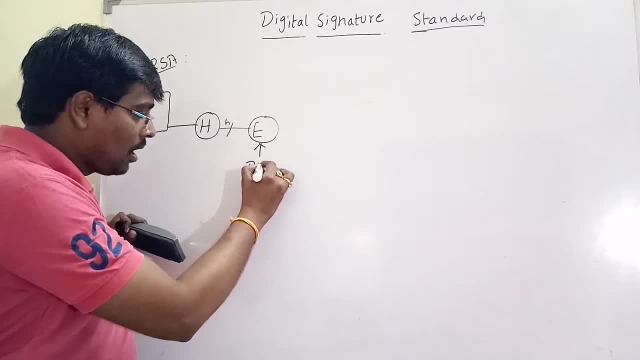 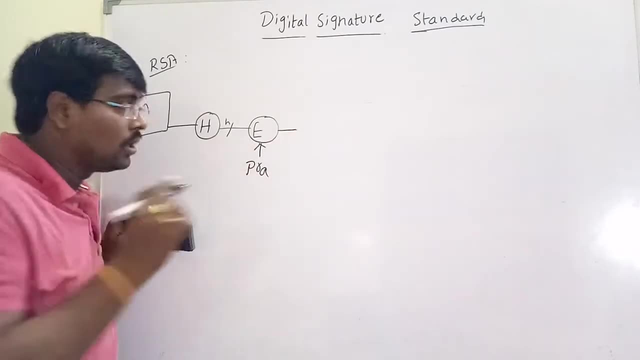 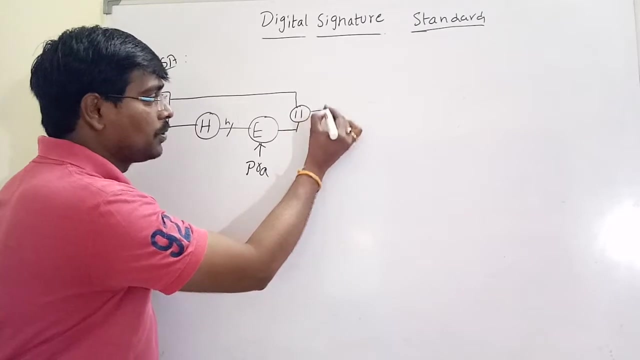 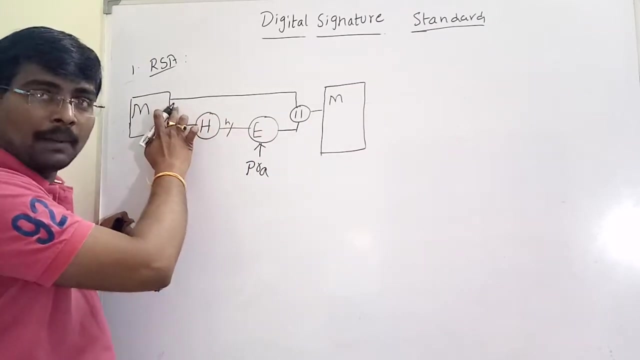 By using private key of a encryption. By using private key of a, It produces some encrypted value. Now this value is combined with this one. Appending this one, It produces What it produces: The message M, Because I am not applying any operation on M. 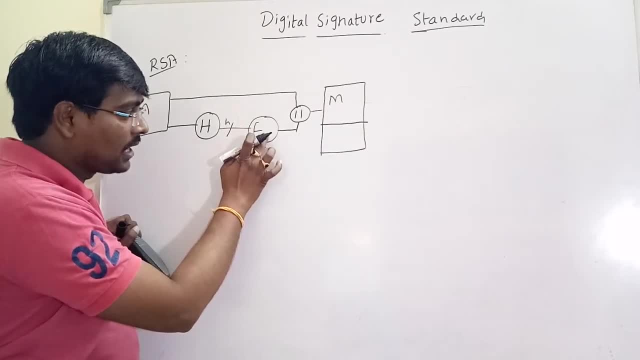 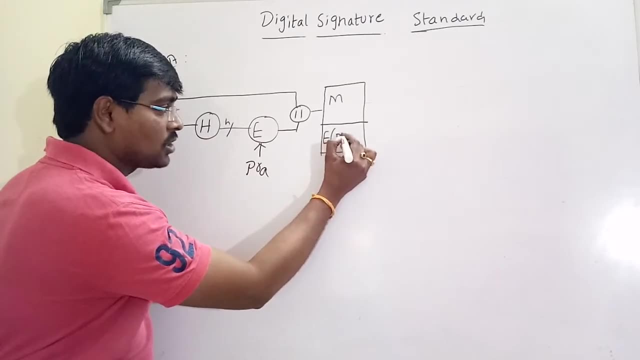 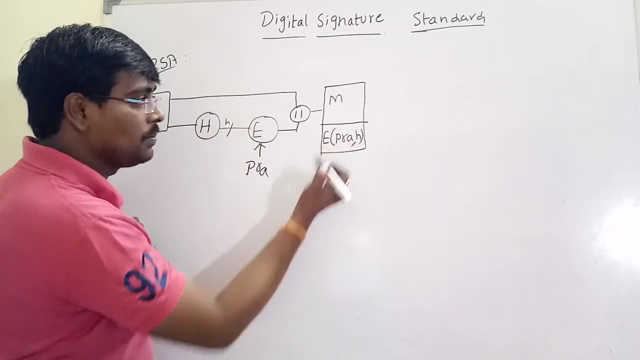 Directly: M is copied And I am performing encryption operation on this hash code. Encryption operation On this hash code By using encryption operation. By using Hash code means some hash By using private key, The reverse procedure. This is at the sender side. 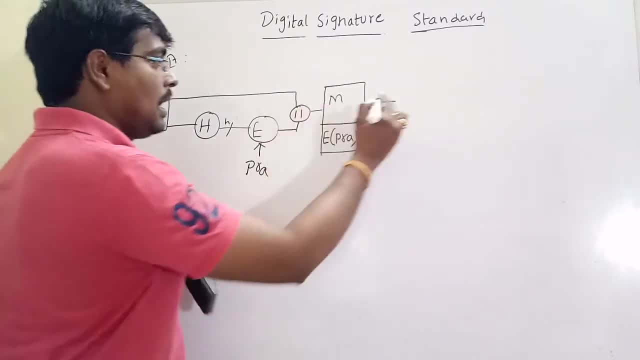 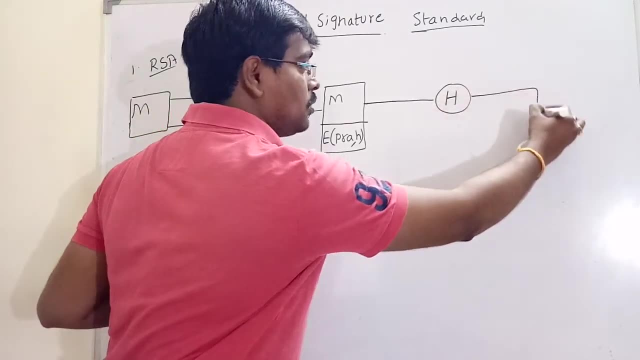 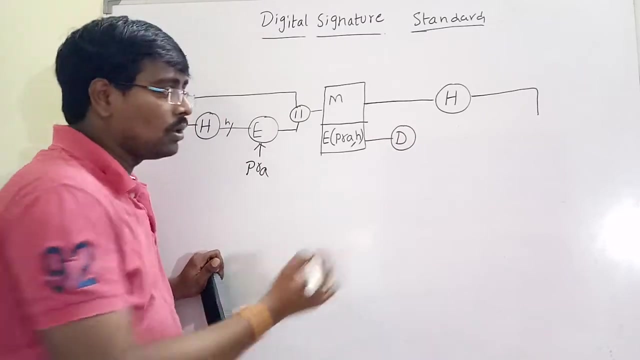 What we will do at the receiver side. Receiver side, simply On the message: I am applying the hash function. I am applying the hash function. It produces some hash code. This hash code is compared with The decrypted hash code. Suppose the decryption is performed. 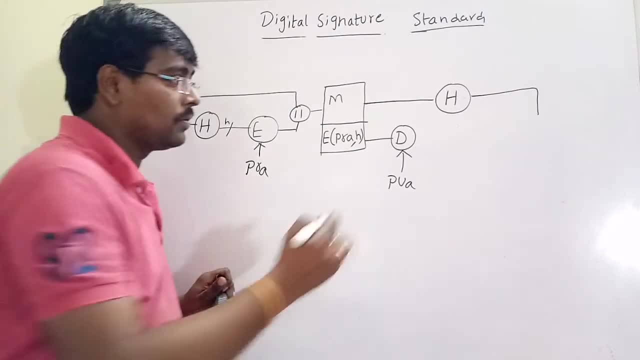 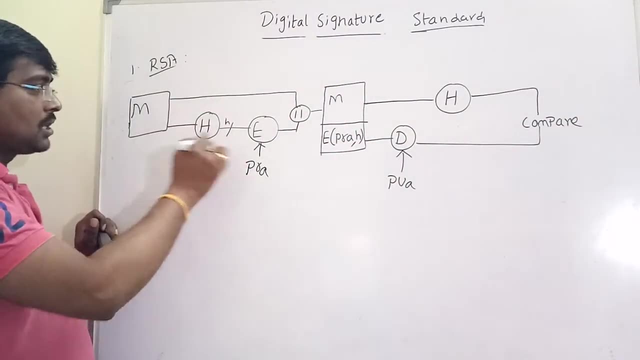 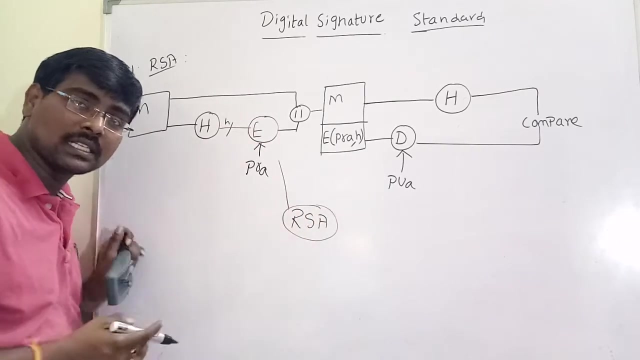 By using public key of a If it also produces compare If these two are same. So in this approach Here encryption algorithm is RSA algorithm. We already discussed asymmetric key cryptography- RSA algorithm. Here the encryption is done by using RSA algorithm. 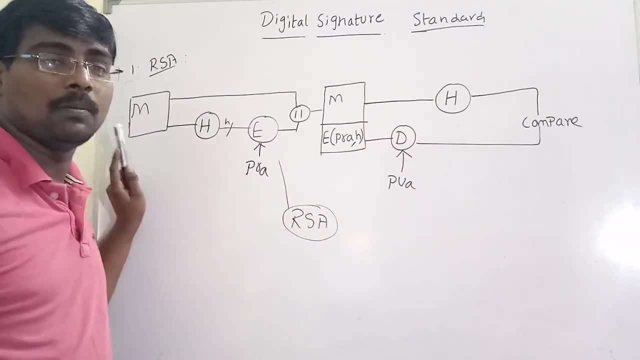 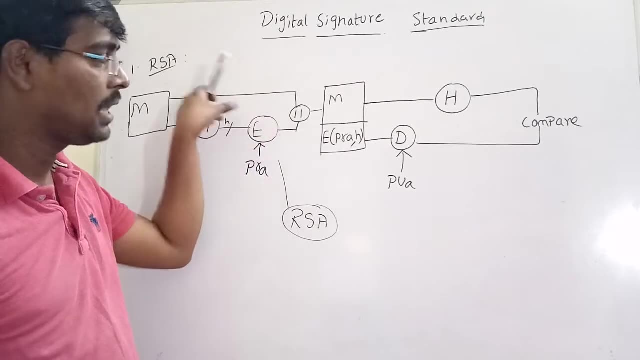 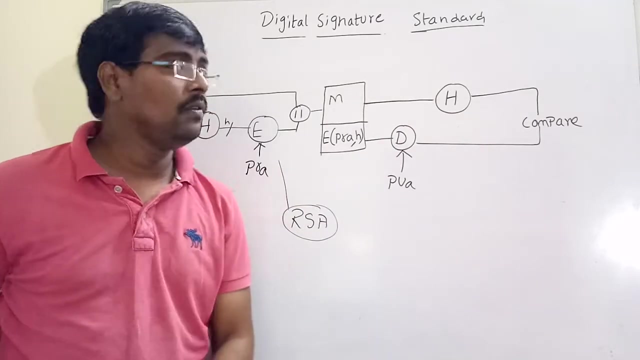 RSA algorithm. This is called RSS approach. RSA approach for digital signature. Okay, We are performing encryption on the hash code And simply append the original message to the Encrypted hash code. Perform the same operation. Now we will move to. 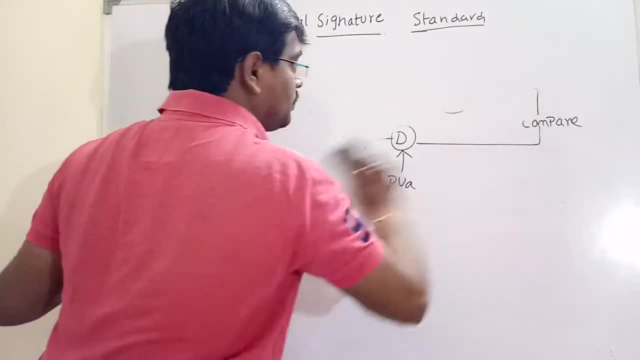 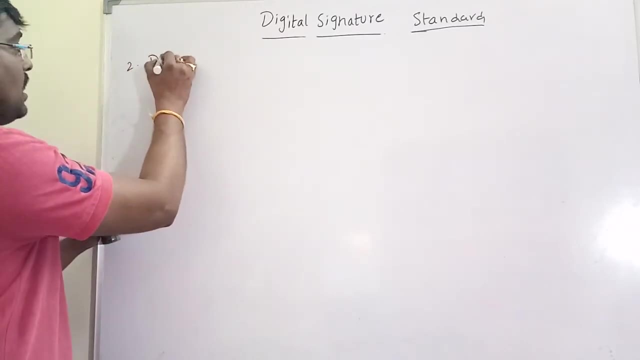 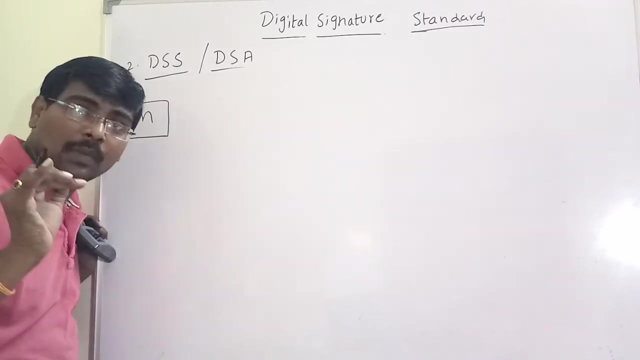 Digital signature standard. Now We will move to Digital signature standard, DSS Or DSA, Digital signature standard Or digital signature algorithm approach. In this approach, First the same procedure Message. So for the message m. 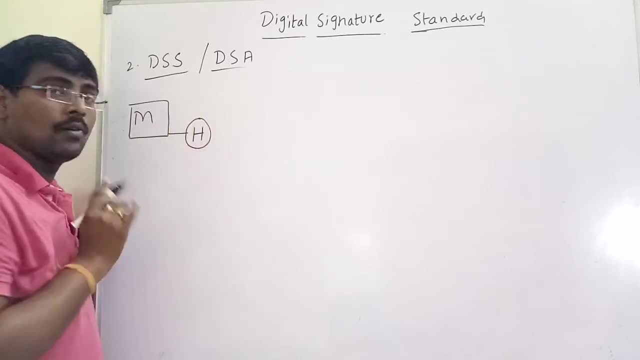 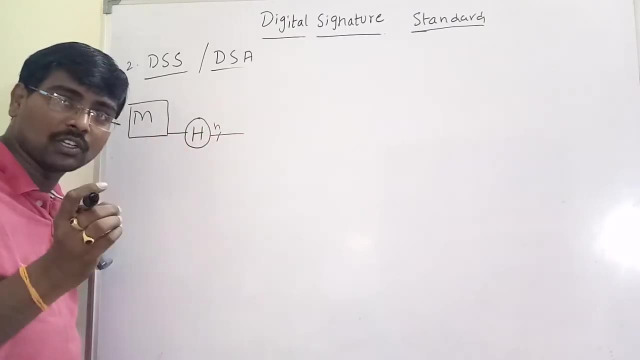 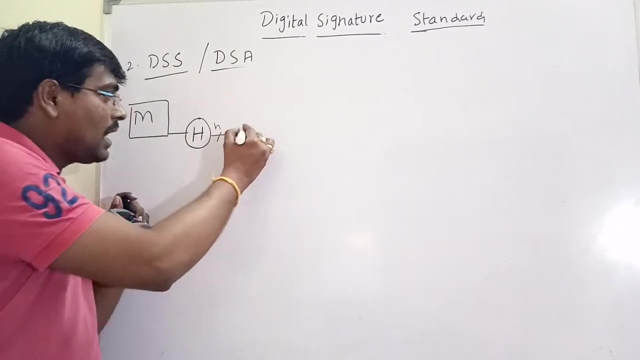 Perform hash operation. Message m: Perform hash operation. After performing hash. Here h means some hash function, Either SHA-1 or SHA-512.. It produces some hash code. Now that hash code is applied to, That hash code is applied to. 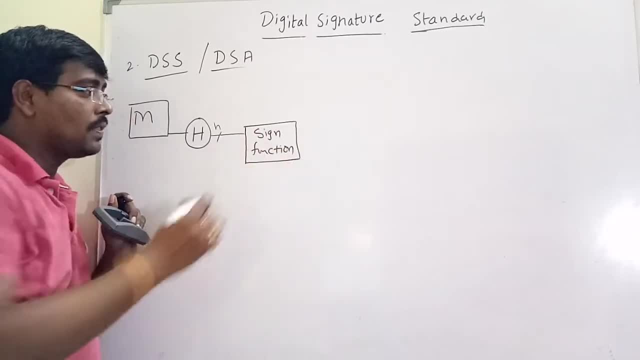 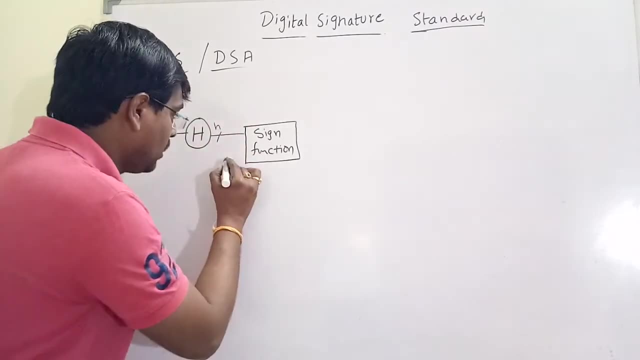 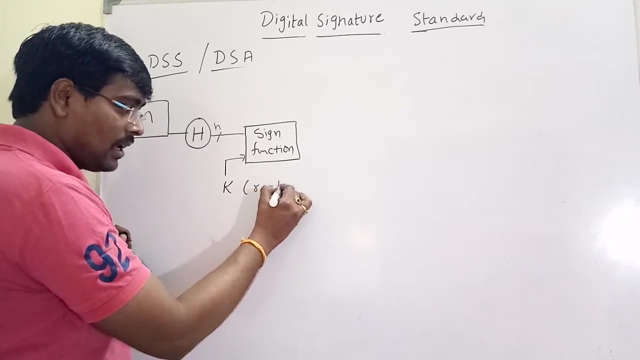 Some signature function. The hash code is applied to Some signature function. For the signature function. What are the inputs? The hash code h, Suppose K, K- any random variable And k is Not the key, K is Any random variable. 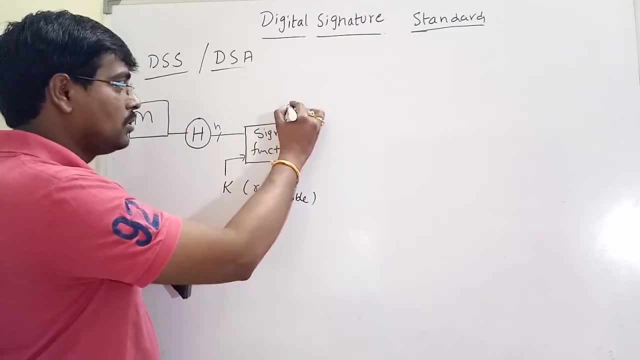 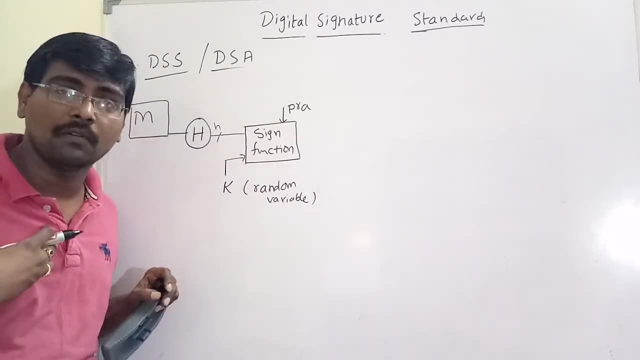 And also What we have to produce: The private key of a. The signature function means: In this signature function, I am performing encryption. In this function, I am performing encryption. For this, I am producing input As a private key of a. 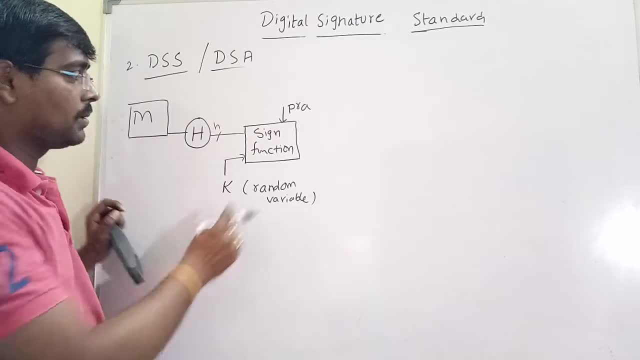 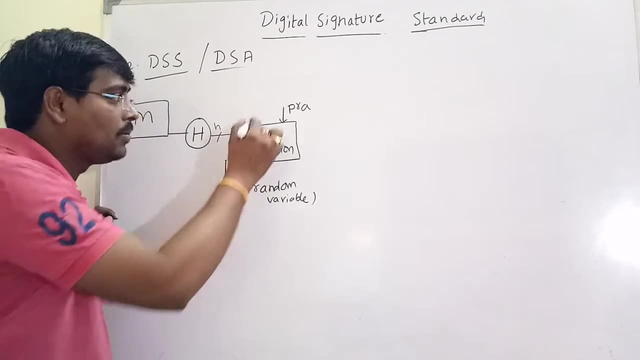 And hash code And any random variable And along with Some g. g is Any global variable And along with Some g. g is Any global variable And along with Some g And along with Some g. 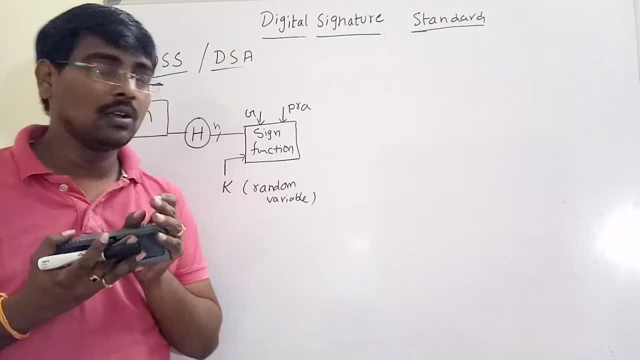 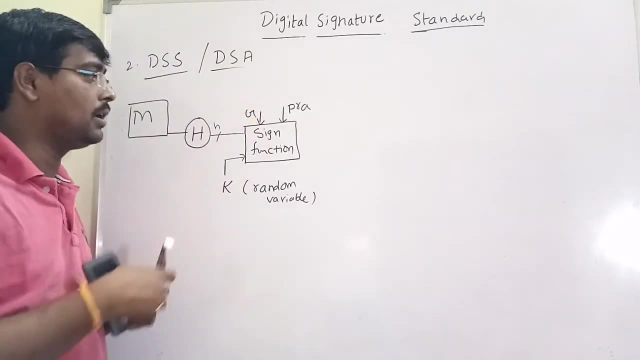 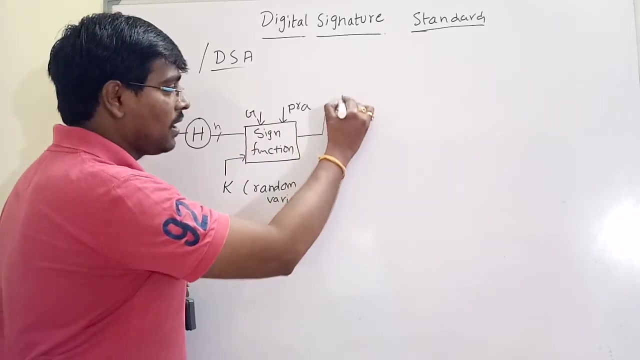 g is Any global element. g is Any global element. Generally, Global means It is a public. So Generally g is Any public Global Element And It produces Some value. It produces Some value. 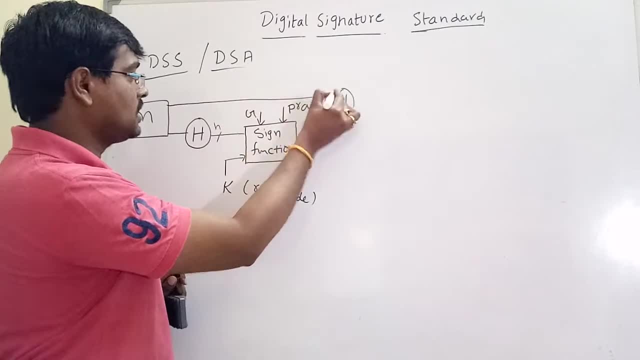 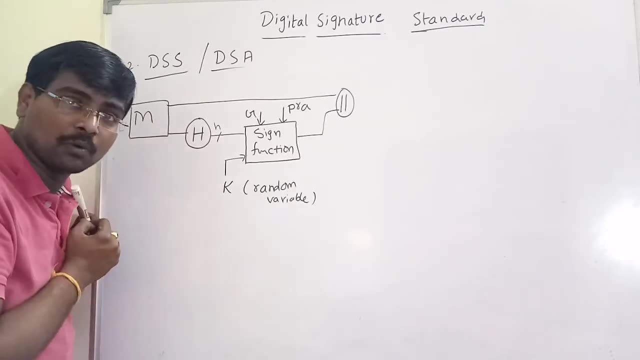 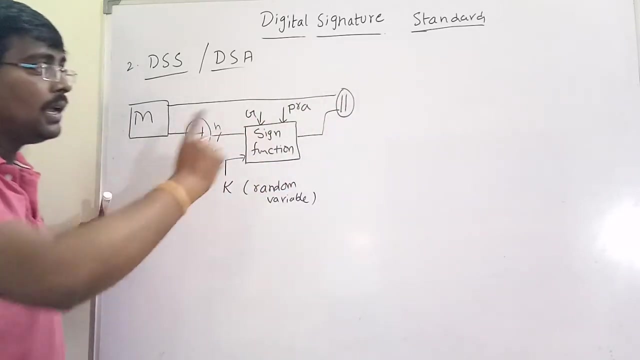 This value Is Appended To The original message Y. Okay, So Similar to RSA, Similar to Previous approach, I am Applying Encryption And Now Append The code In This. 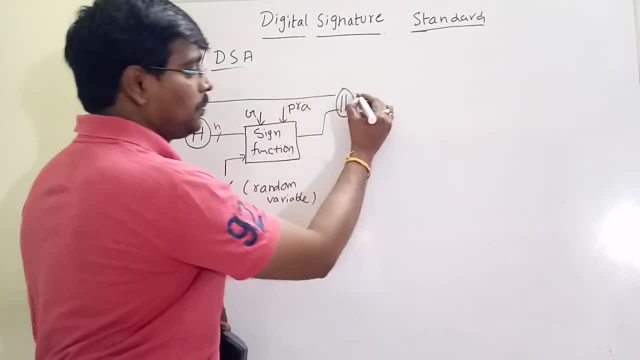 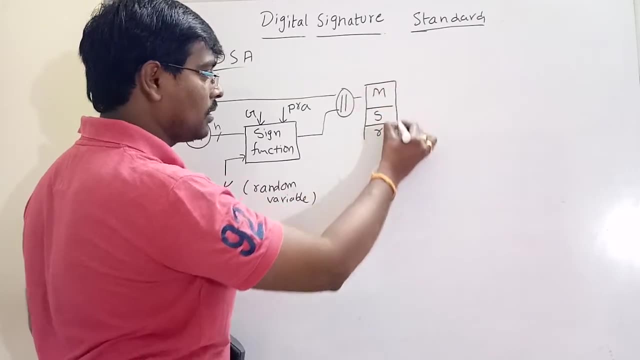 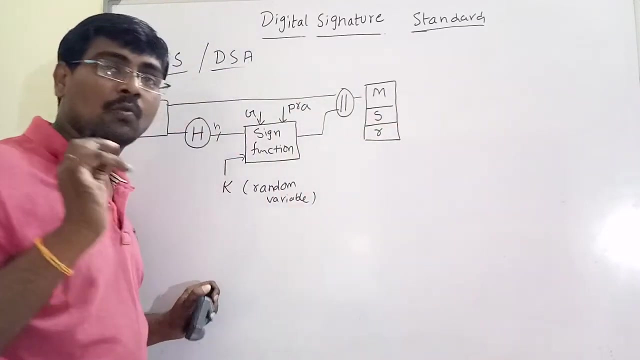 DSS Approach. I am Using Signature Function. We will Discuss What Is Signature Function Letter. It Produces Three Parts: M, S, R. This Is Applied To. 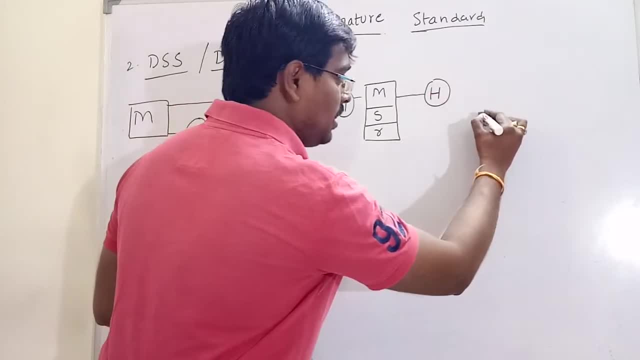 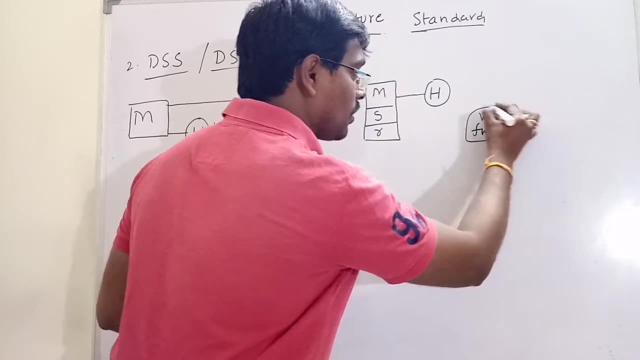 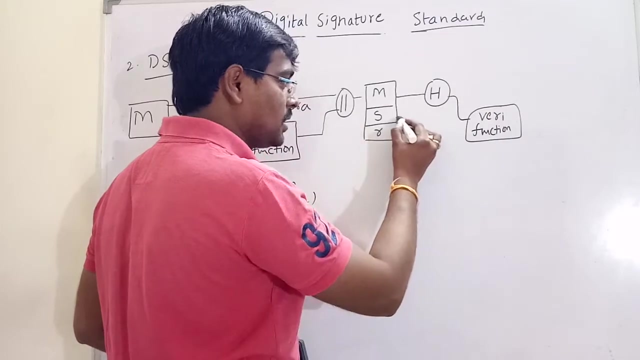 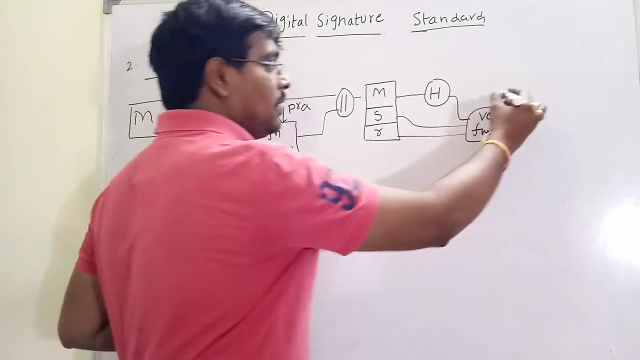 Hash Function, The Same Procedure, The Reverse Procedure. This Is Applied To Hashing And Here We Are Using Some Verification Function. Here We Are Using 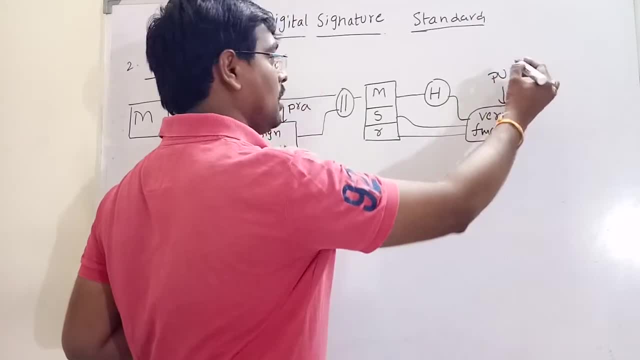 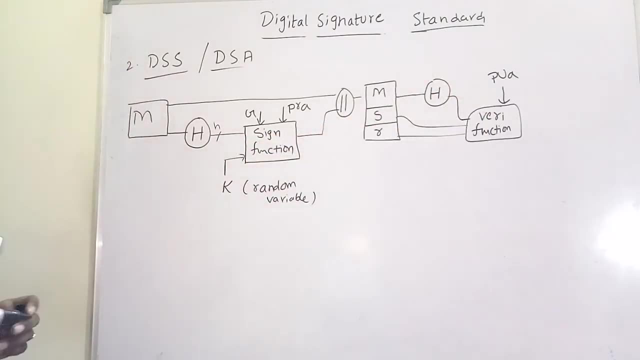 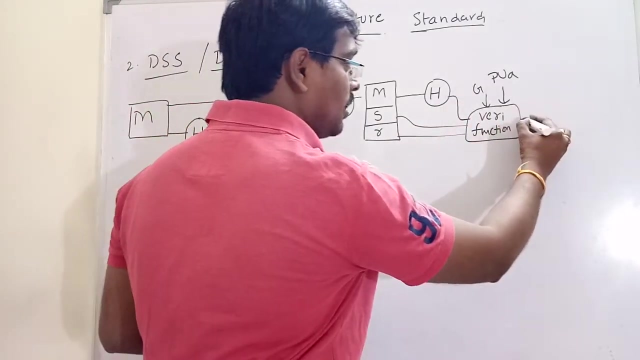 Verification Function. One Of The Input Is A Public Key Of A. If You Are Encrypted By Using A Private Key, Compulsory The Decrypted. 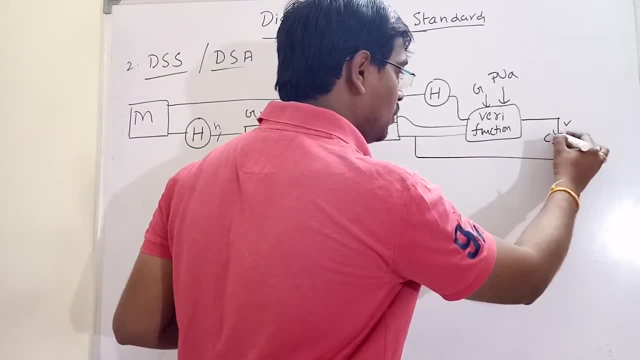 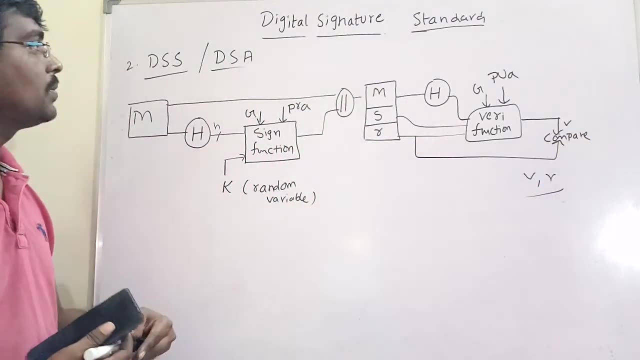 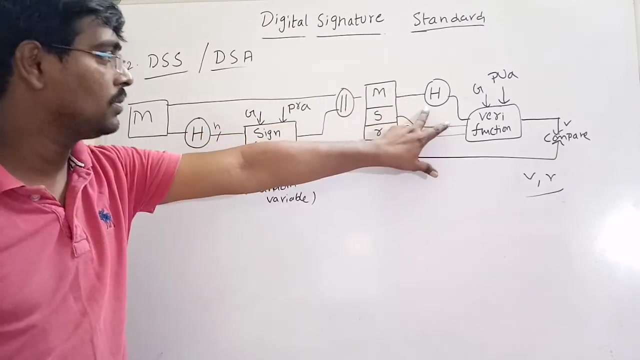 By Using Public Key Of, That Is V Comma Or R Compile. If Both Are Same, Our Algorithm, That Is, Encryption And Decryption, Is Performed. 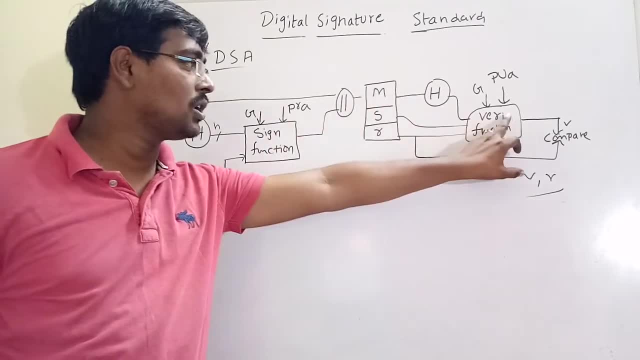 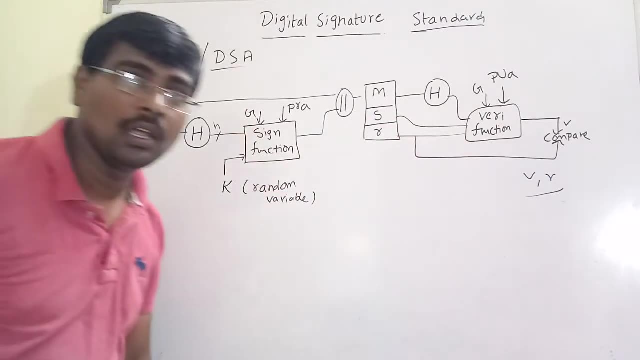 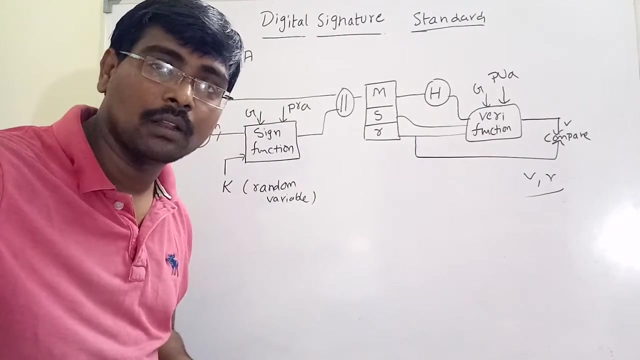 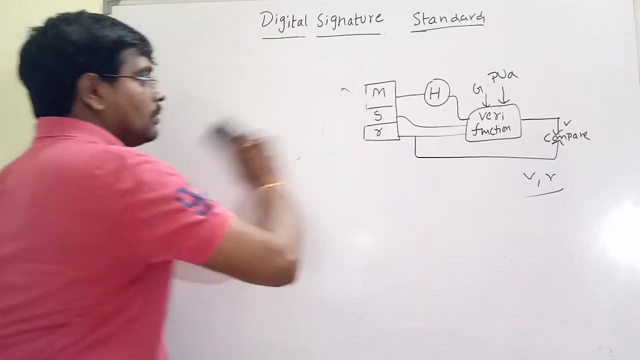 Successfully. Okay, First, To The Original Message: Apply Hash By Signature Function. Now We Will Discuss Each And Every Parameter In Detail. So In This D. 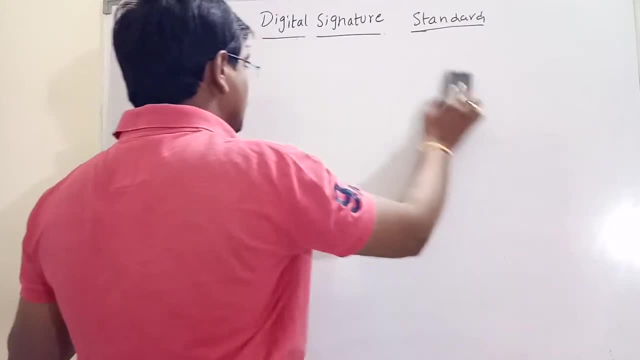 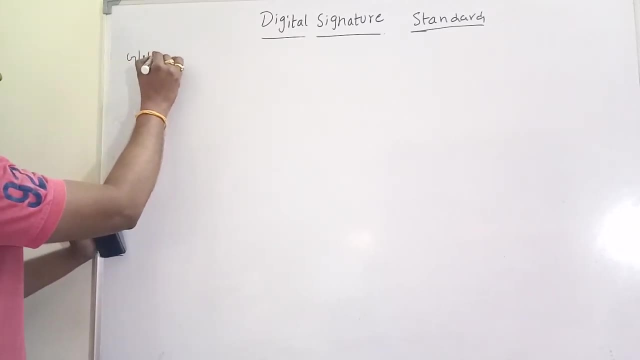 S Algorithm In This D S Algorithm. First, What Are The Global Components? The Global Components Are? We Are Selecting Three Values: P, Q And. 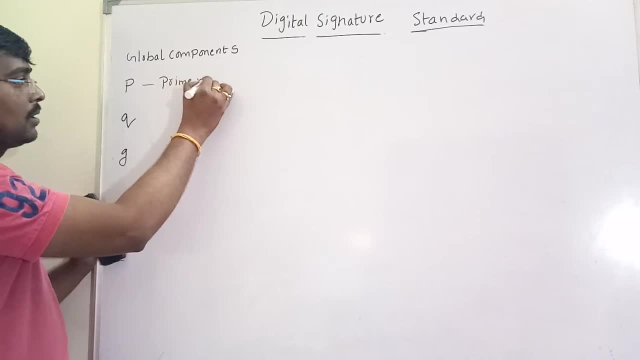 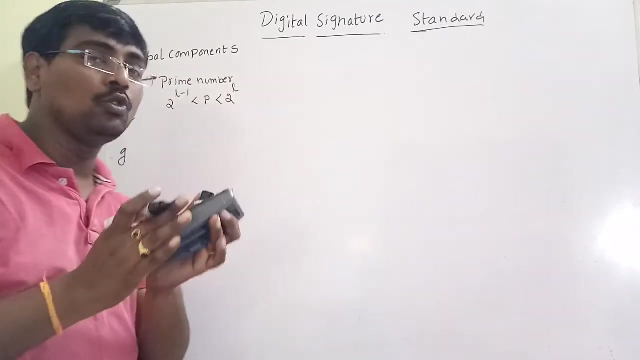 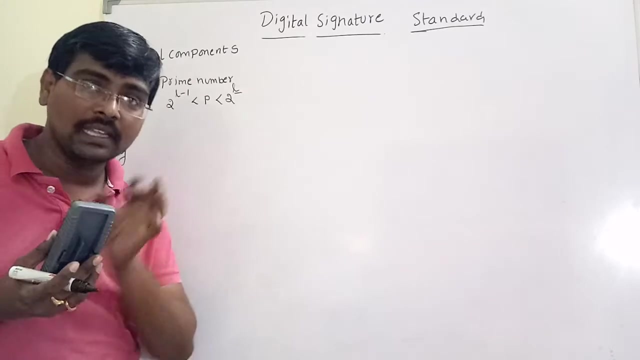 G, So P, Q And G. P Is A Prime Number, P Is Any Prime Number In The Range Two Power L Minus One Two. 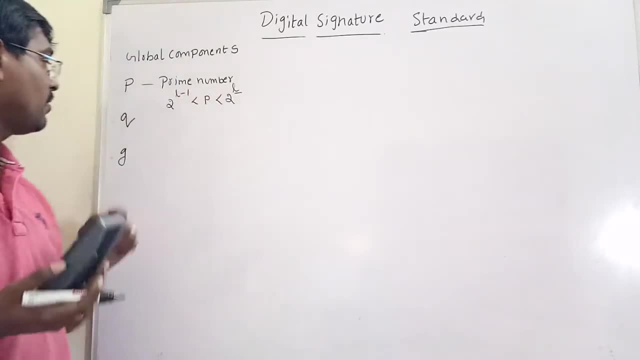 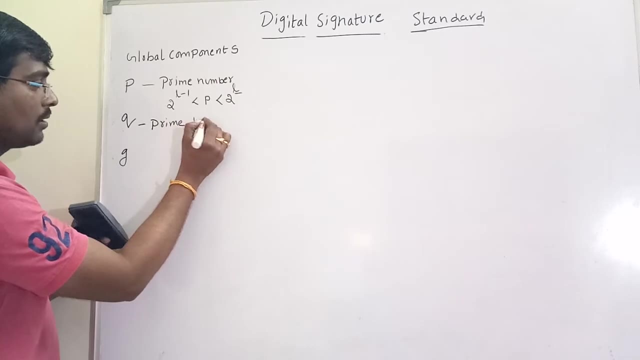 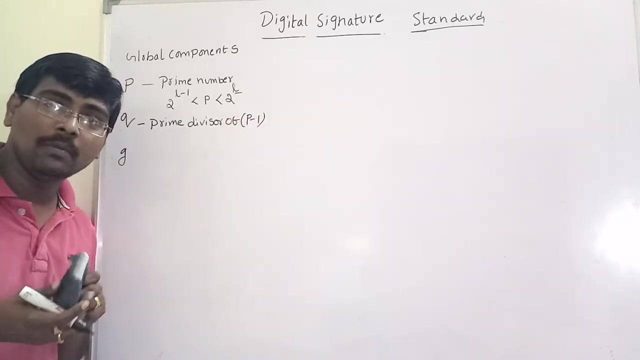 Two Power L. What Is L? L Is The Length Of The Bills. L Is The Length Of Bills. That Is The Synch confidence Of The 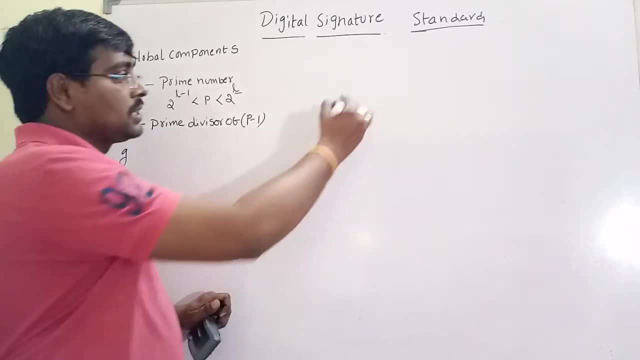 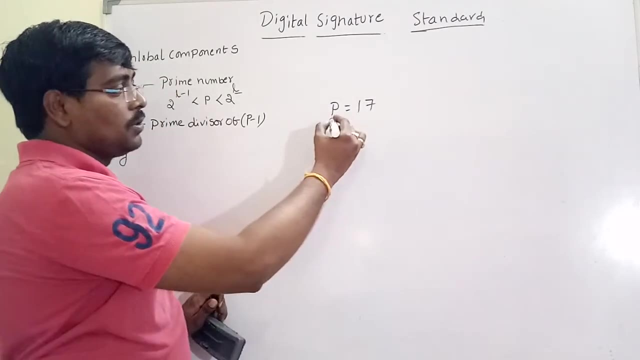 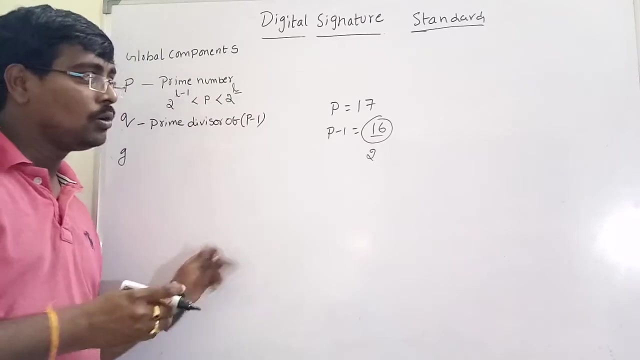 thinkings Can Gill Hold On Even Ten, But The Round Could Be Like Log roadmap. Those Treat You As Like Finding The Thick musun Is. 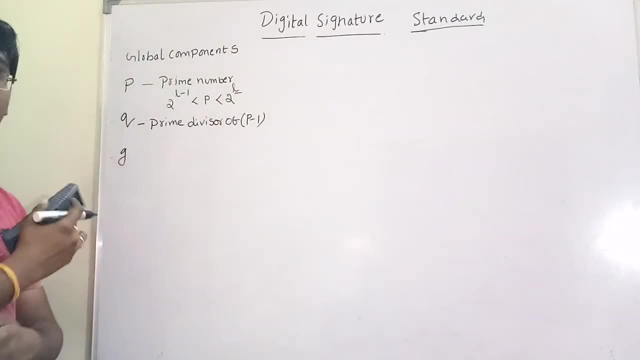 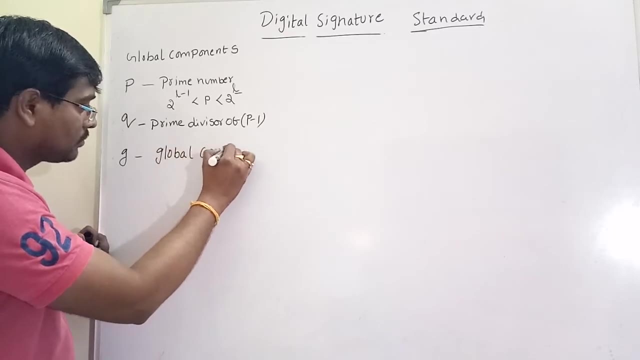 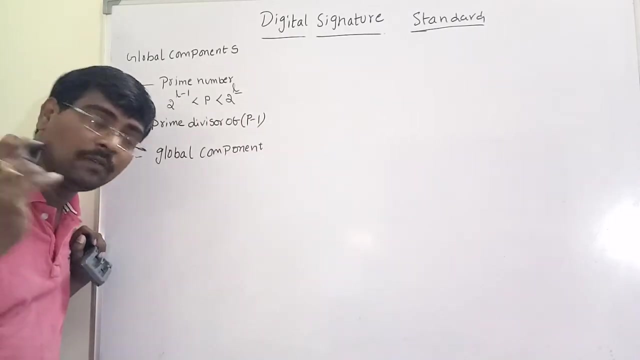 so Q is any prime divisor, any prime divisor, that's the. G is a global component. G is a global component. G is a global component. what is the value of G? H power- H is the hash code we are producing: H power P minus 1 by Q P. 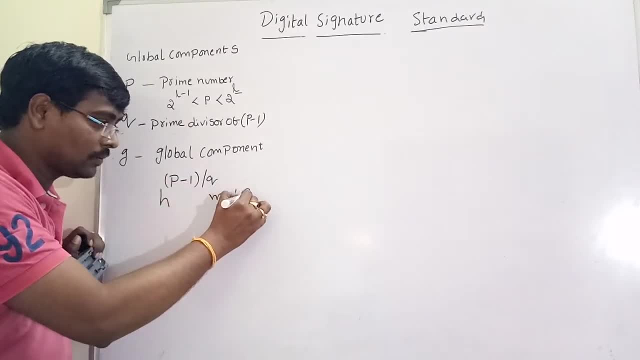 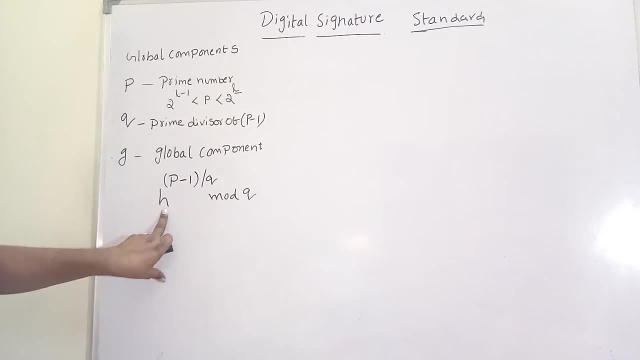 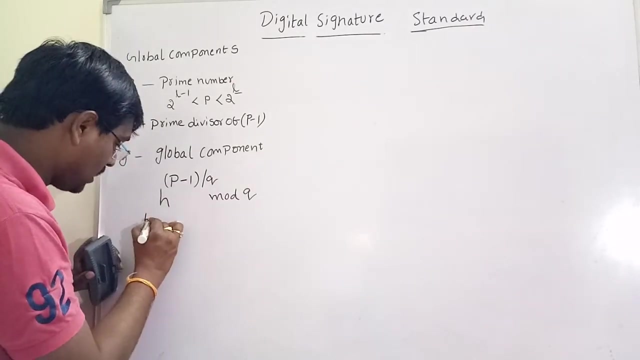 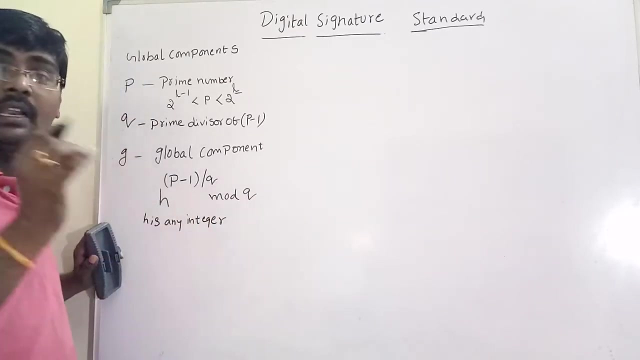 minus 1 by Q mod Q. G is equal to G, is a global component, and the value of G is H. power P minus 1 by Q, by Q. here remember: H is any integer, H is sorry, H is not a hash code. H is any integer in the range 1 to P minus 1, H is any. 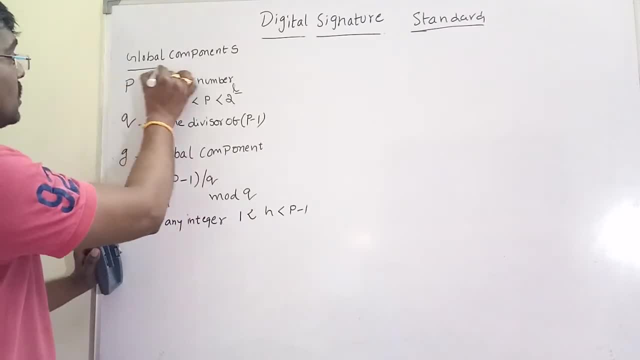 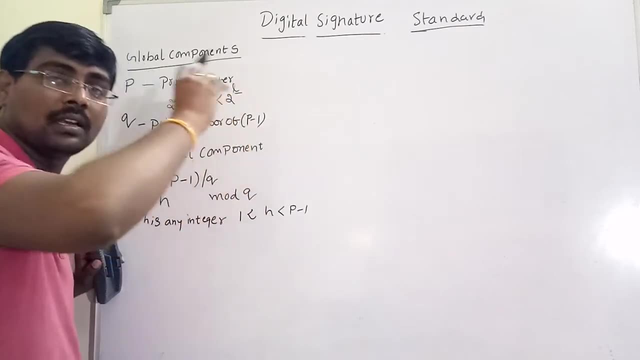 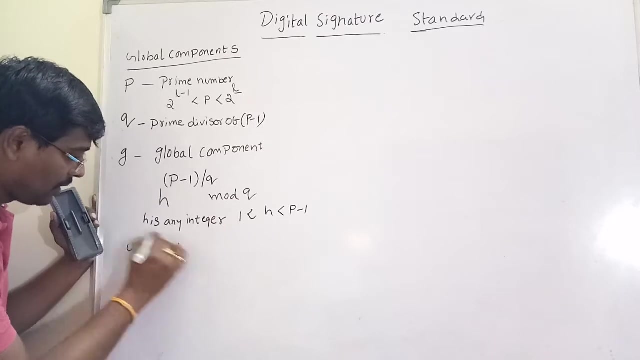 integer in the range 1 to P minus 1. these are global components. global components means these components are used at the encryption side, that is, at the sender side and receiver side. now user private key. the first one is completed. user private key: assume any random variable X. X is assumed as a private key. X is any random number. X is: 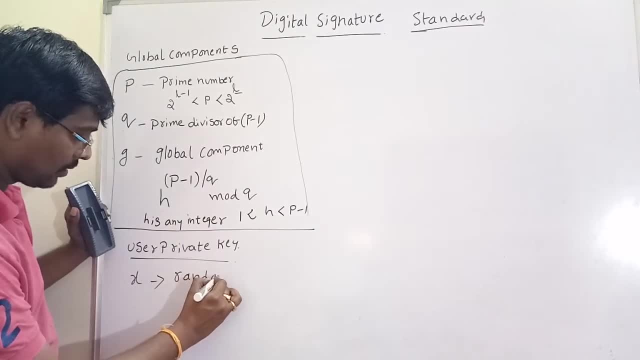 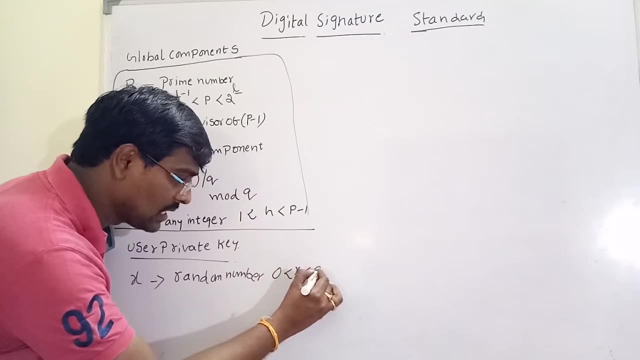 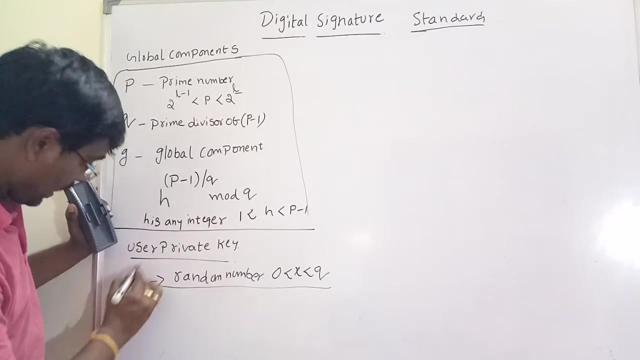 any random number in the range 0 to Q, that is, 0 less than X, less than Q, X is any random number- 0 less than X, less than Q, and user public key. okay, the public key is specific to Hrying. so you take a mention of KEVIN, you take a mention of KEVIN and you take a mention of H doctor and you take a mention of the user. so the user is the public key, so you can开始 theля hu trade back to the user, personal public key and you baking. now h're from sign language there we meet, broken less than. 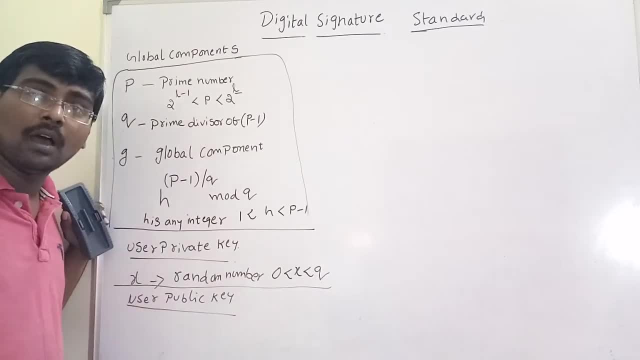 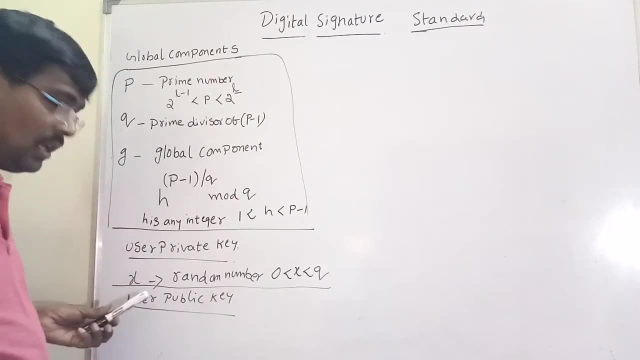 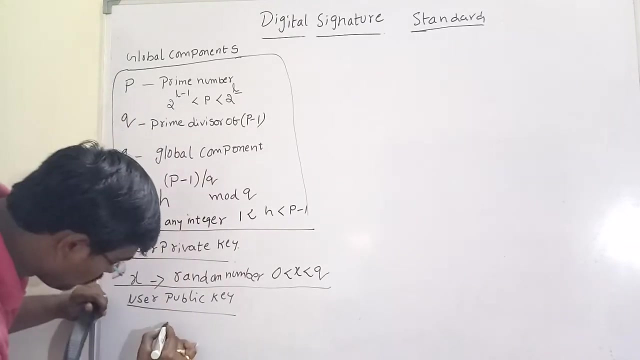 degree. so you meet only x- manually. hgil, that means really you leave as a key. okay this, okay the public remember always: the public key is calculated by using the private key. you assume X is the private key, Y is the public key. the public key is calculated by using the private key X. so the value of Y is equal to G is a. 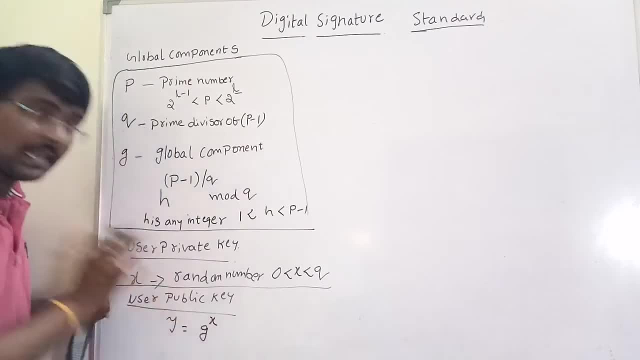 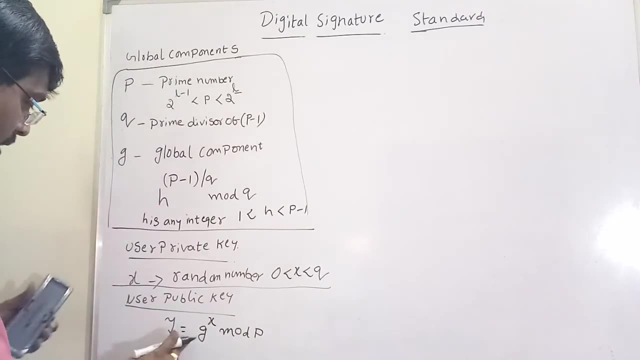 global component: G power X. X is the private key mod P. so the public key is Y is equal to G power X mod P. G power X mod P. this is the public key. so today we are discussing with the global components P, Q and G. user private key X. 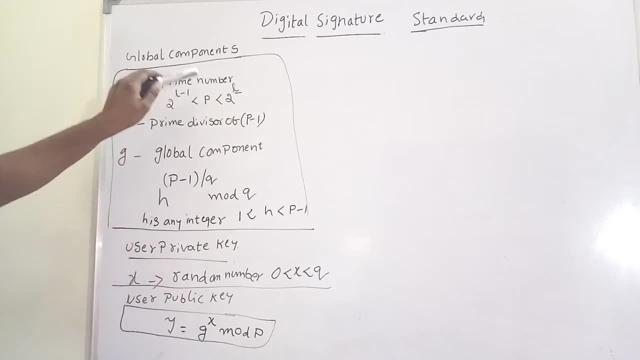 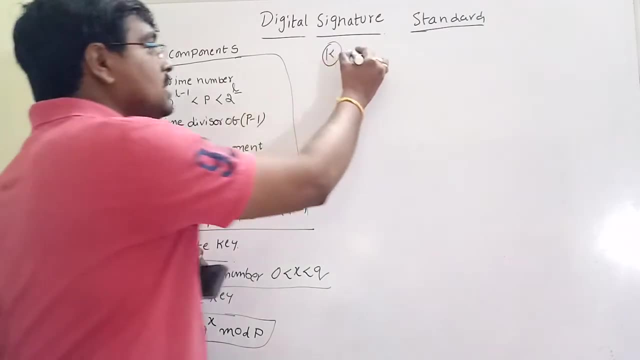 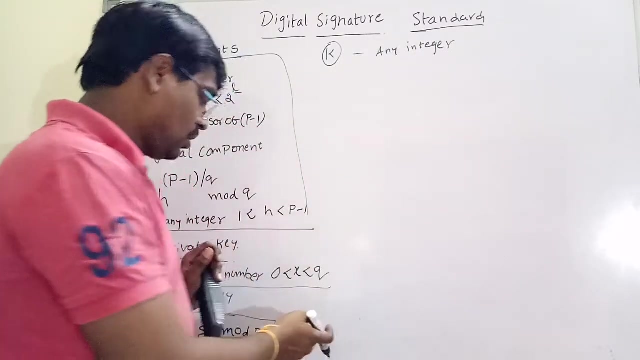 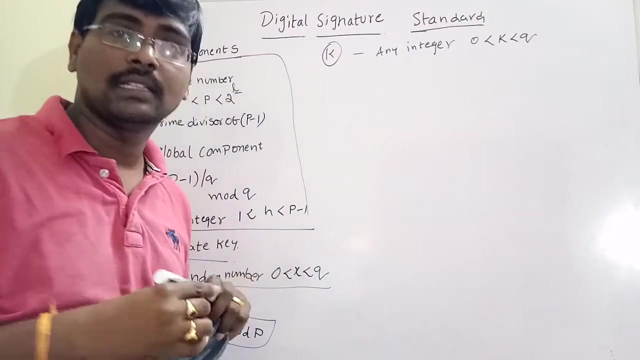 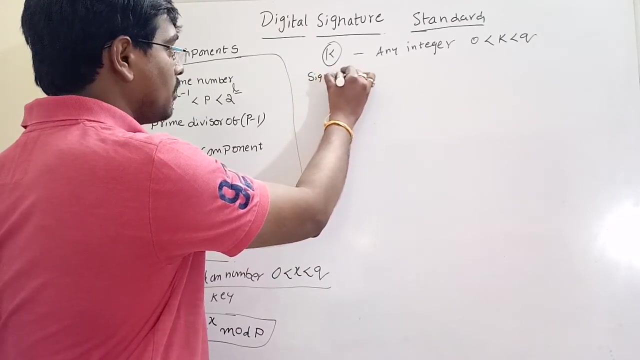 and user public key Y. in example, we are in the session 1mo, K. Suppose the K is any integer in the range 0, less than X, less than Q. so now signature component. so you're can avoid more. asegas d式. you think you naac внимание, it's enough, you can't avoid more. I don't concentrate the more flour. show off with the clock, really, but I show it down the window because the play is in the middle of this analysis. follow with a chunk and every one of these changes will forever stop. 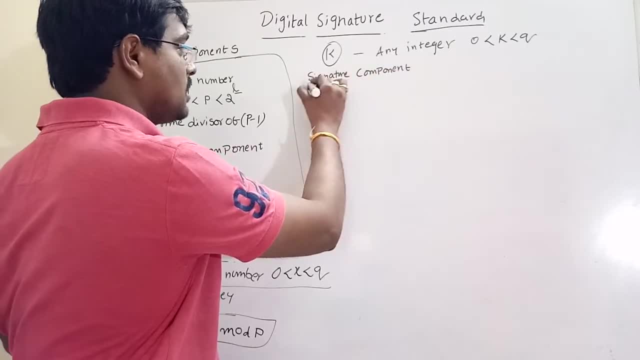 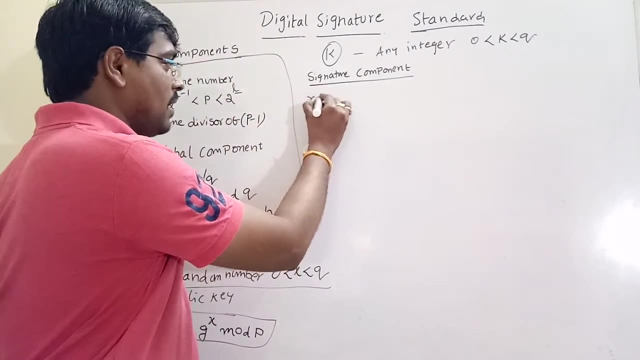 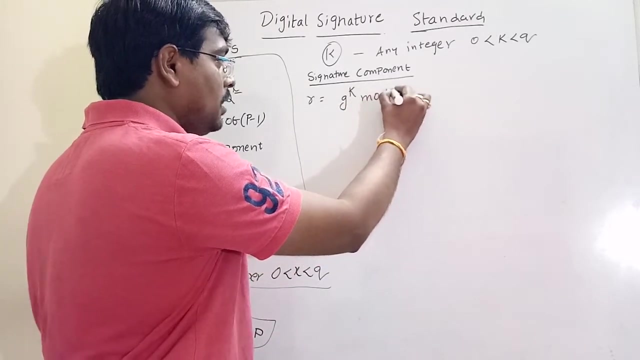 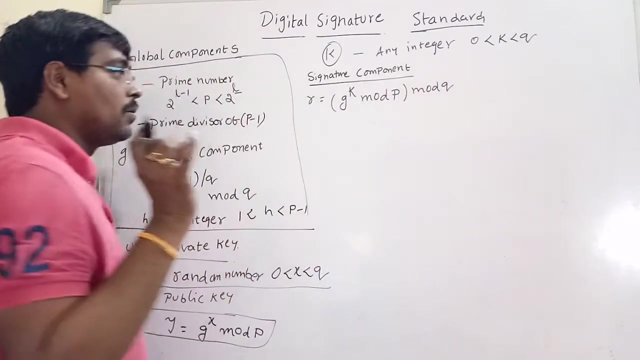 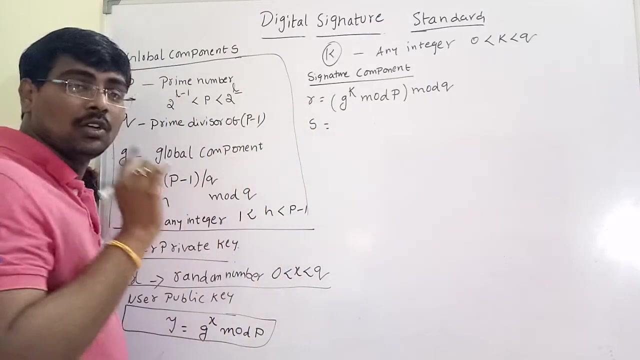 we already discussed the signature function. The signature component contains two terms. One is r and n1 is s. So s and r. Suppose the value of r is equal to g power k mod p. g power, k mod p mod q. g power k mod p mod q. This is the value of r And s is equal to k. inverse k is any. 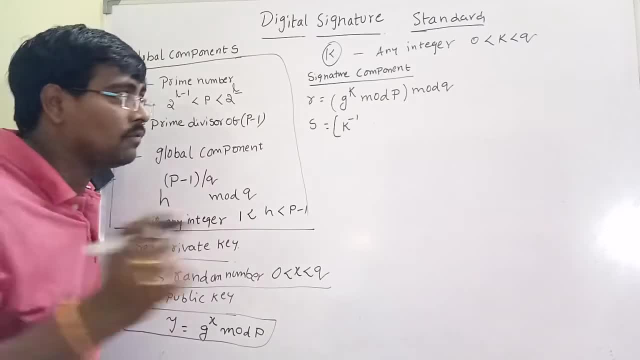 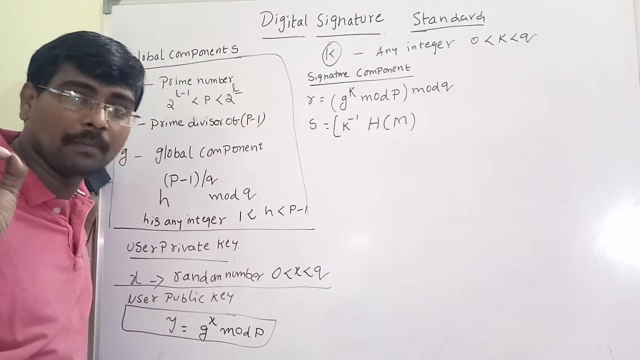 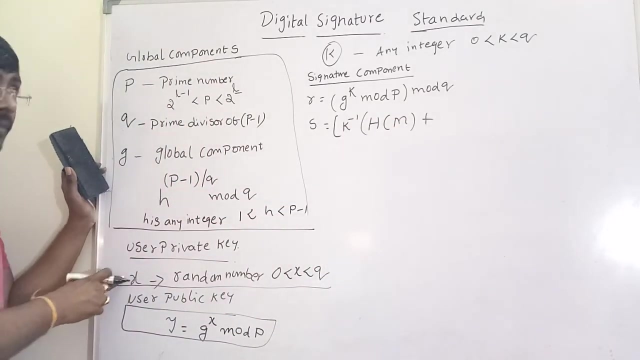 integer in the range 0 to q. k. inverse h of m. h of m is hashing of m. h of m is hashing of m plus X is the private key. X is the private key. R is one segment, X into R, S is: 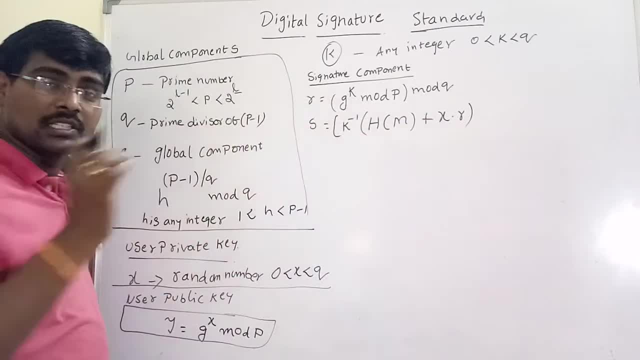 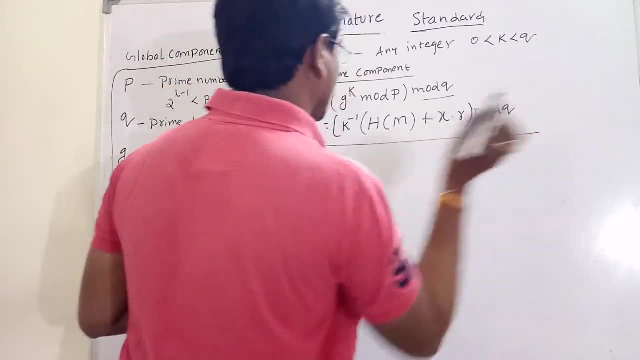 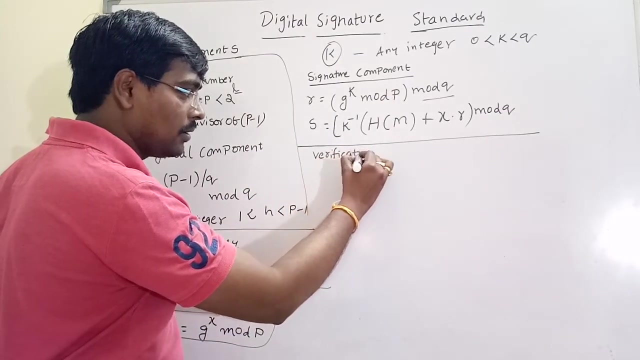 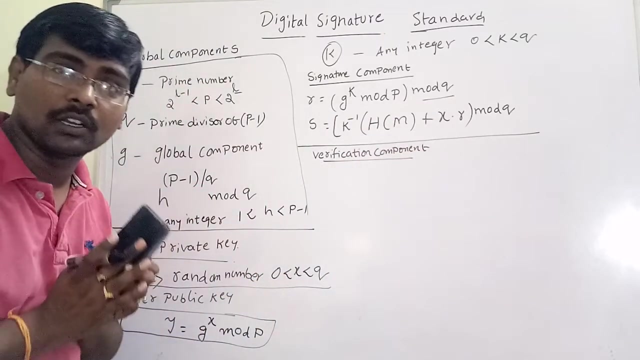 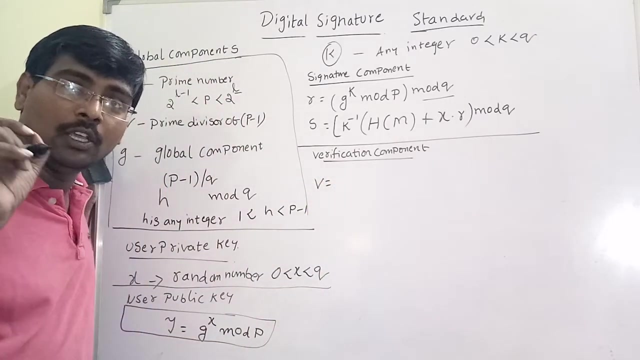 equal to K, inverse H of M plus X into R. similarly mod Q. this is the signature component. this is the signature component and finally the verification component. finally, the verification function. the verification component is the verification function. V is equal to G power U 1, G power U 1. so what are the? 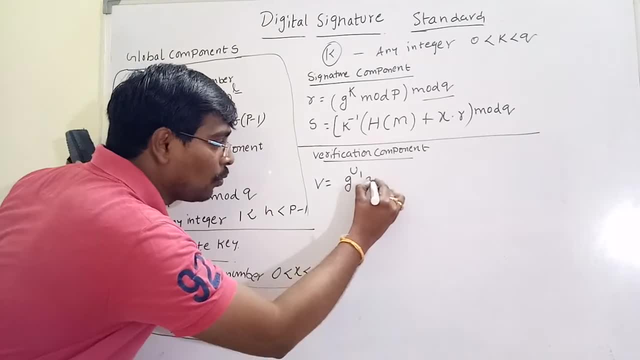 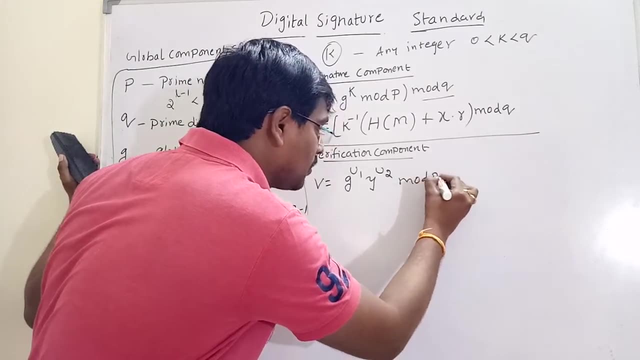 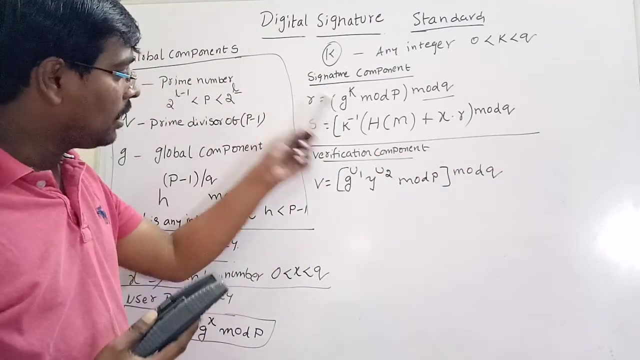 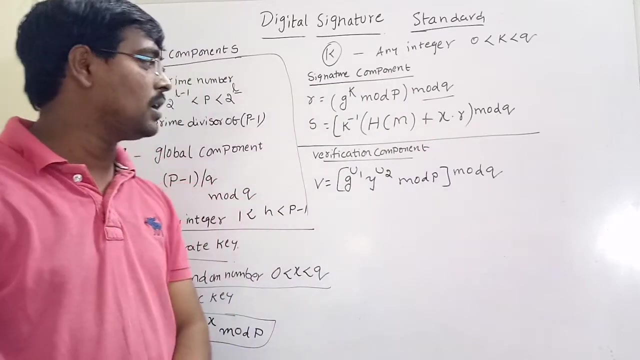 values of human when you write letter: G power, U 1. Y power U 2. G power: U 1. Y power U 2 mod P, mod Q. ok, remember, in all the terms Common Term is G. G is the global component that is at the sender side and receiver side we are using G. 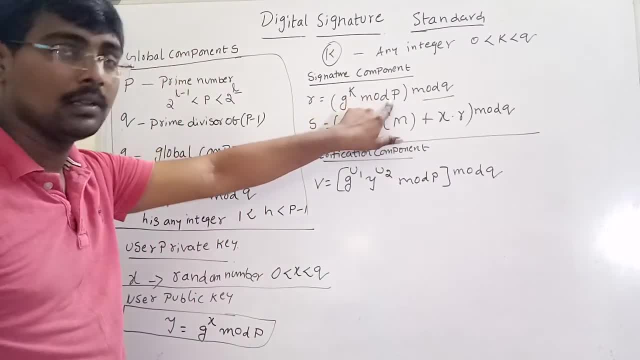 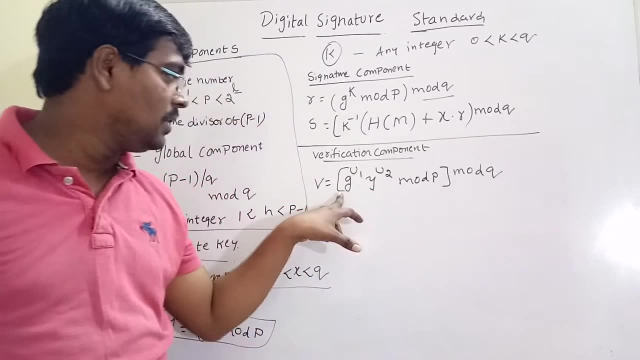 see this one: G power K mod P at this sender side, suppose at the receiver side, after verification function we have get the value V. so V is G power mod P, suppose some. another term is Y G power L is equal to G power K mod P. 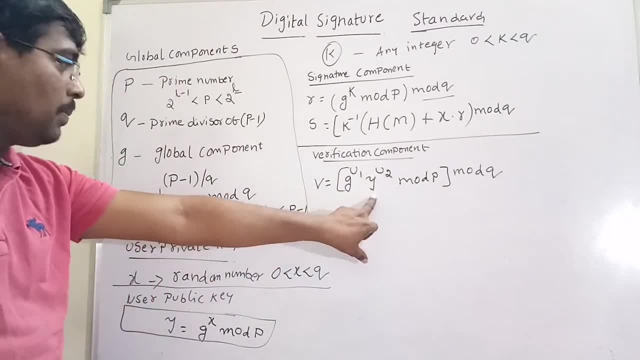 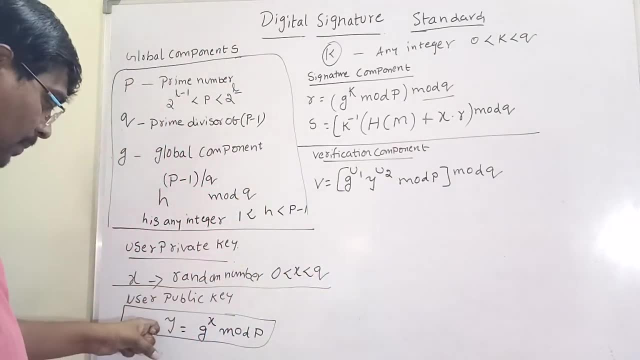 power U1, Y power U2 mod P. Here Y is the public key. At the receiver side we are performing verification by using the public key of A, So the public key is Y. So Y and G are both are global. Y and G, both are global. Now we will write what are the values of U1. The 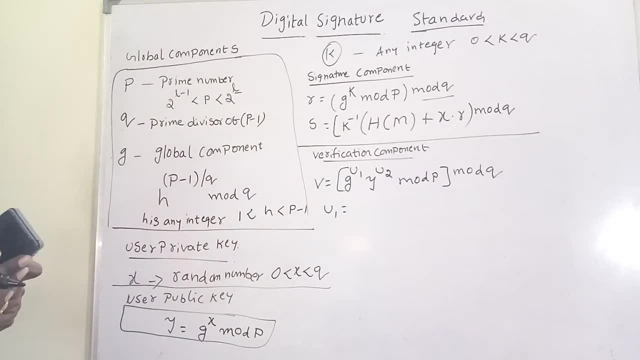 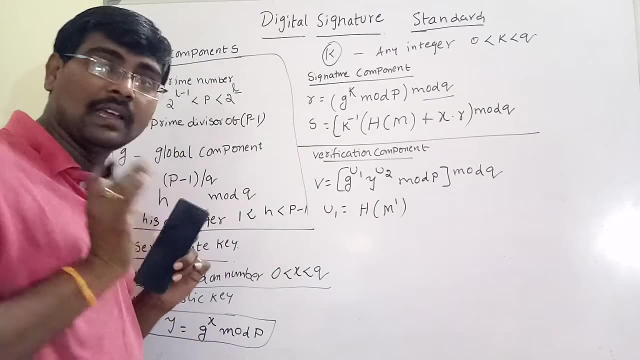 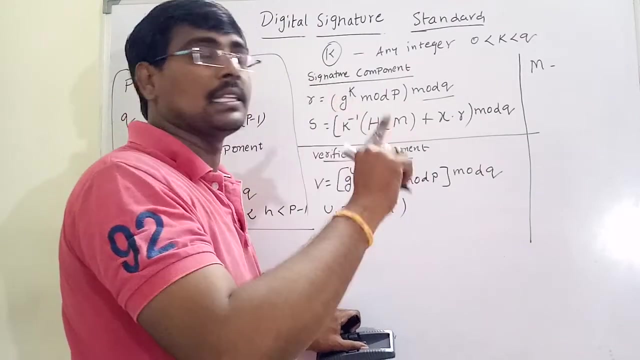 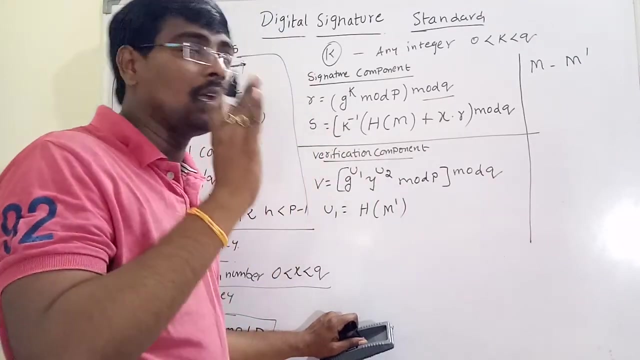 value of U1 is H minus H of M1.. What do you mean by M1?? Suppose M is the message at the center side. The same message, simple notation- is M dash at the receiver side. Just my assumption is M dash is also the message. This is at the center side, this is at the receiver side. 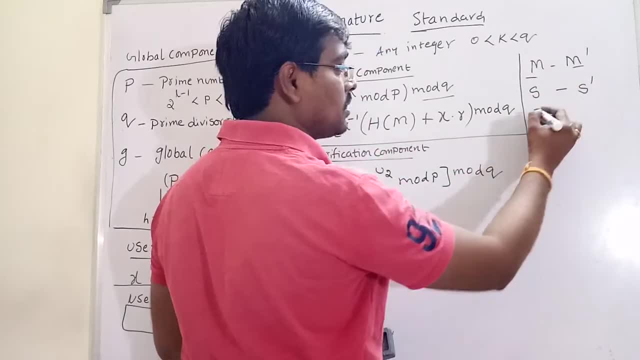 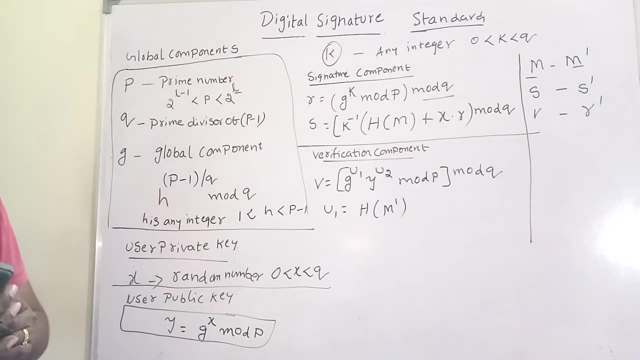 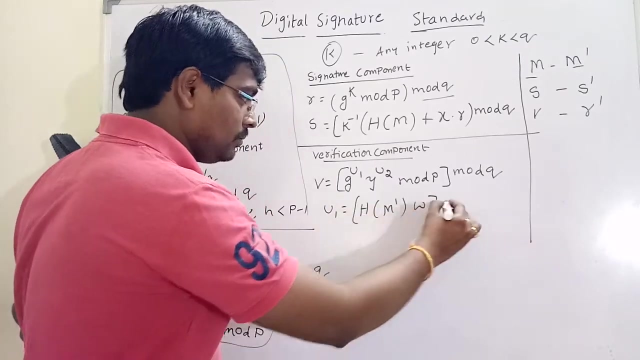 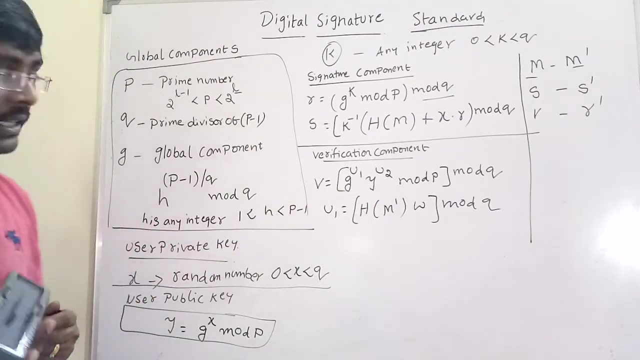 Suppose S is at the center side, M dash is at the receiver side, R is at the center side, R dash is at the receiver side, Just to differentiate between sender and receiver. To differentiate between sender and receiver I am using the dash into mod Q, H of M dash, W, mod Q. What is the W here? again, M dash means. 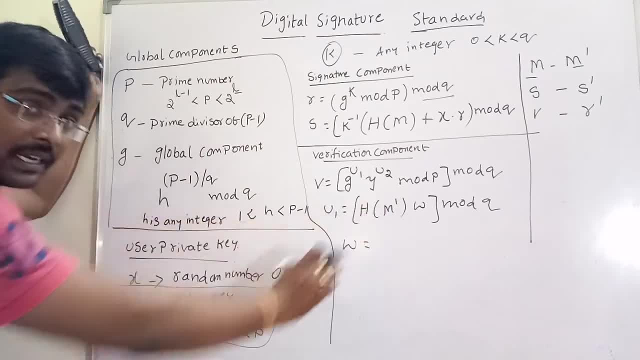 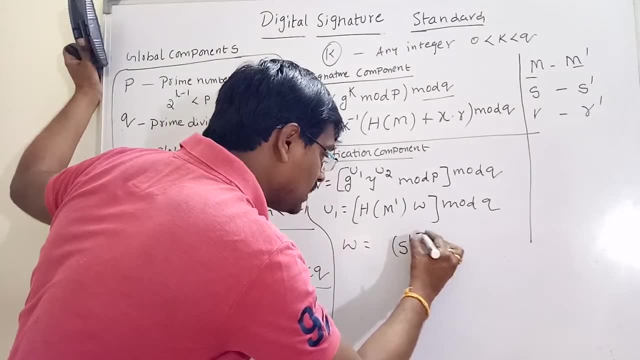 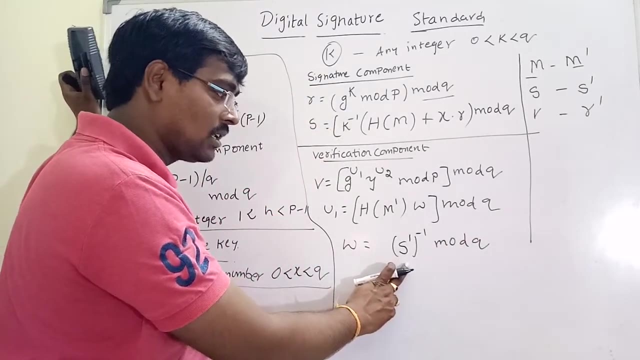 the same message. H is at the same site. the receiver side M dash means the same message at the receiver side. Suppose W is S dash inverse. mod Q: The S at the receiver side is represented as S dash. at the receiver side S dash inverse. 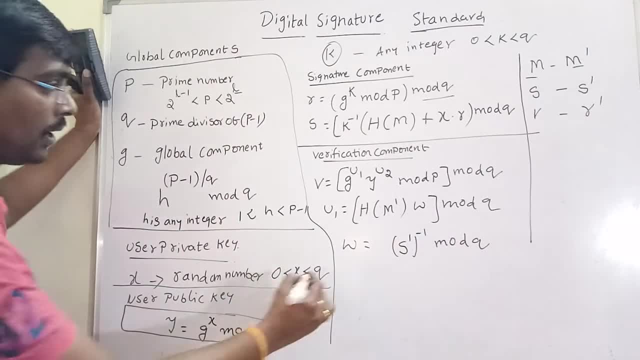 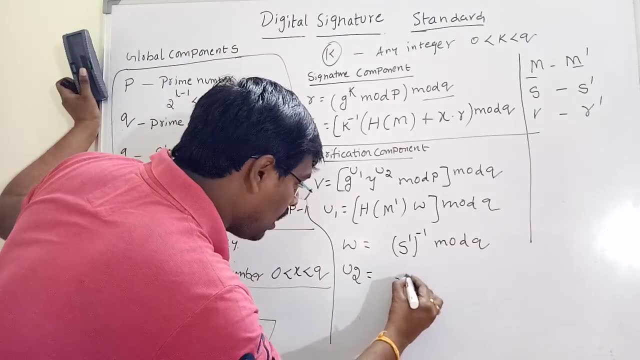 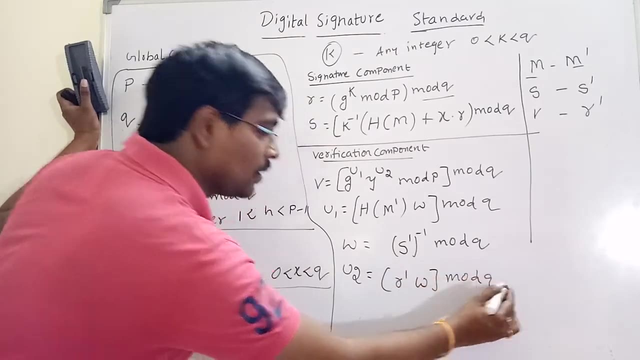 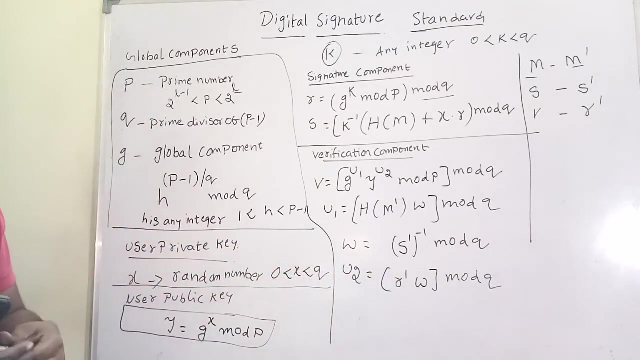 mod Q. This is the value of W, And what is the value of U2?? U2 is equal to, similarly, R dash, R dash. W mod Q. U2 is equal to R dash, W. R dash is the value of R at the receiver side. W mod Q. 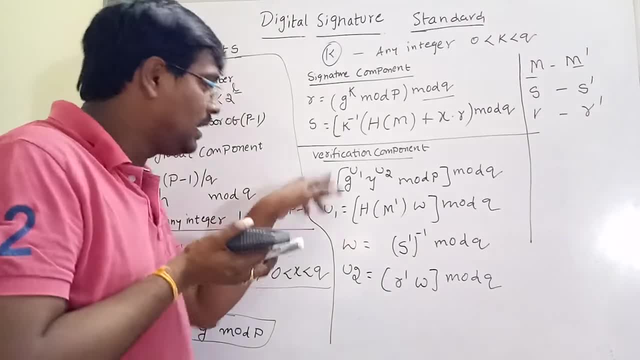 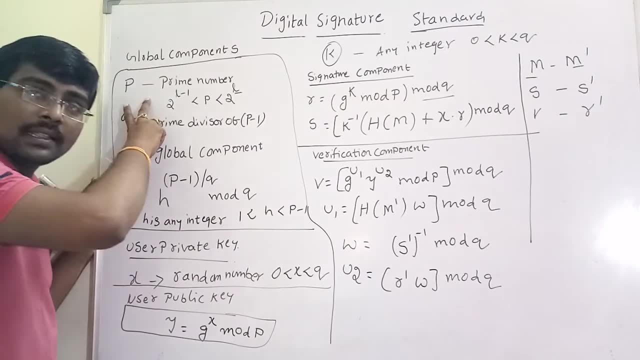 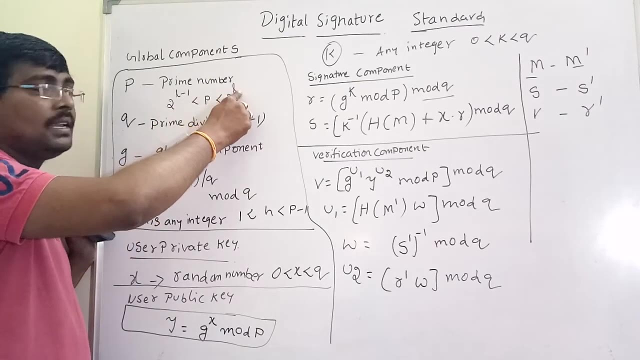 And finally, if the value of V and R dash are same, that is the discharge signature. So this is the final algorithm. Initially we are taking three parameters: P, Q, R. P is any value in the range 2 power L minus 1 to 2 power L. Here L is the length of the wheels And Q is the prime. 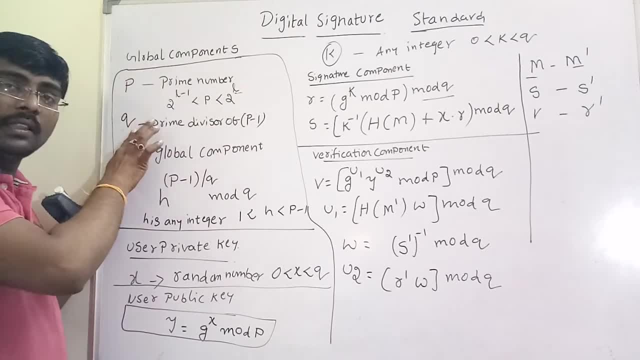 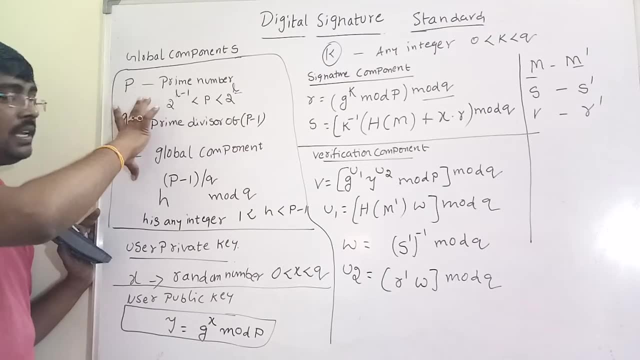 divisor. If you know the value of P, definitely we can get the value of Q. Q is any prime divisor of P minus 1.. G is any global component Here? these three values are your assumption. These three values are your assumption. G is any global component. The formula for calculating: 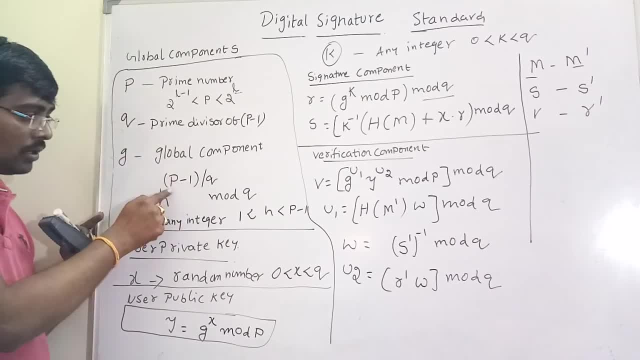 G is, if you know the value of P and Q, Assume any integer, H. Assume any integer is your choice: H power, P minus 1 by Q mod Q, This is the value of G. Once you know the three values, and I am constructing my private key. 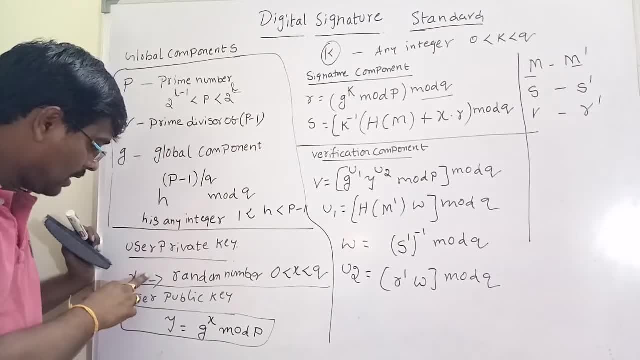 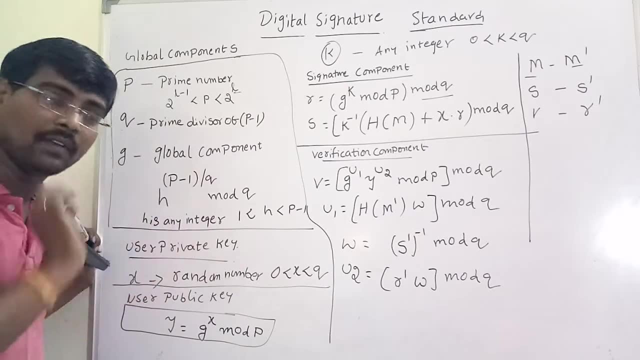 Assume I am randomly selecting X as the private key. In my assumption I am assuming X as the private key. Remember always the public key is calculated by using the private key. So the public key Y is calculated by using this global component and private key. 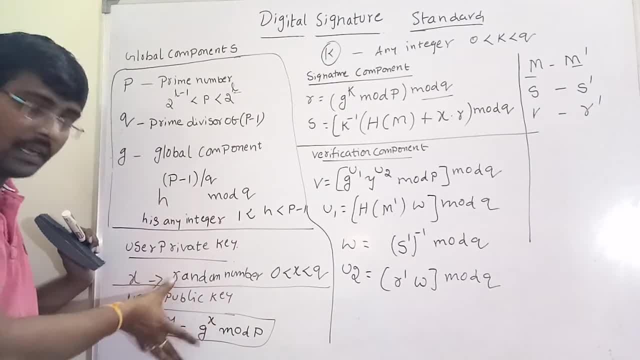 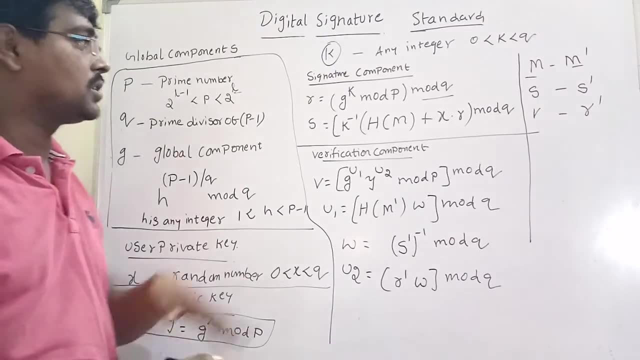 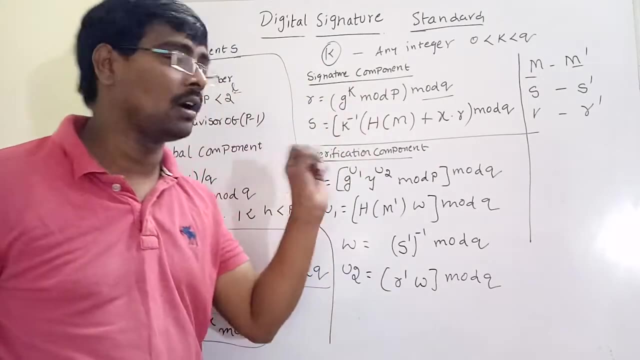 So G power X mod P. So I am knowing my private key and public key. Now assume K is any integer in the range G to Q. We have to get two functions: Signature function and verification function. In signature function we have two terms. One is S and another one is R, Suppose 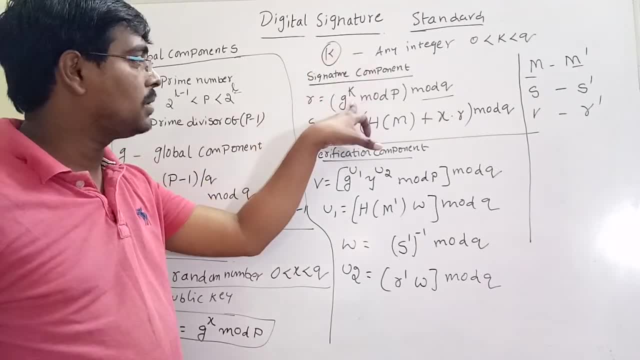 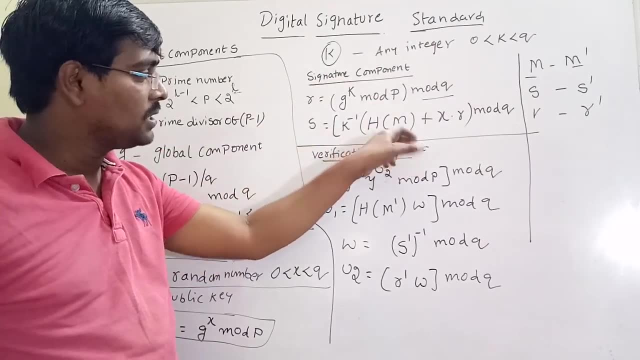 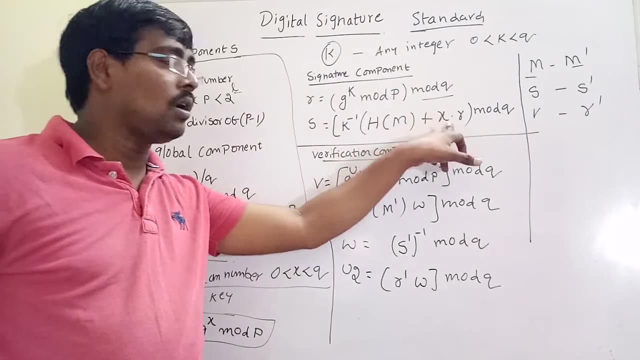 our formula is here. we are assuming K, any random number, G power, K mod P mod Q And S value is K. inverse H of M means hashing On the message M plus X into X is the private key into the value R mod Q. This is the value.